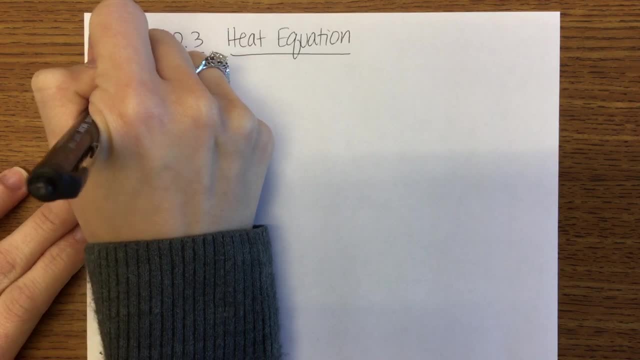 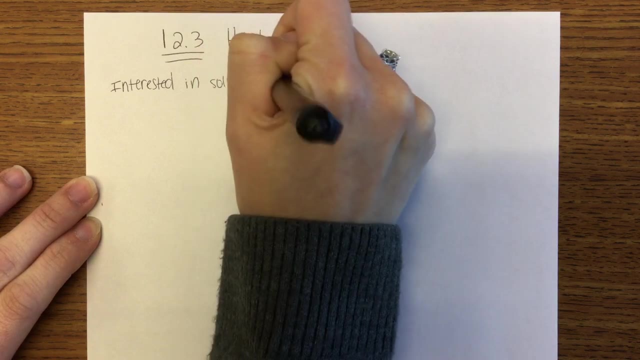 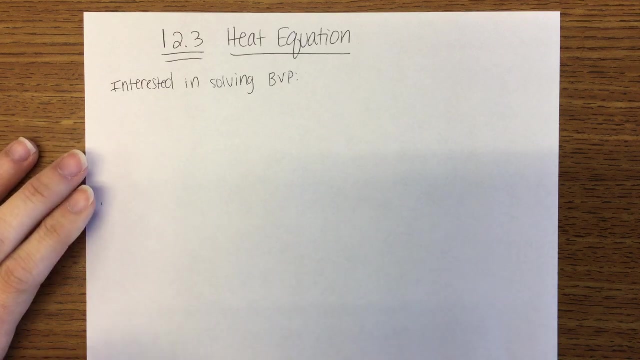 Okay, so, like I said, we're interested in solving the heat equation. We are going to be solving a very specific form of the heat equation. So, again, a heat equation is just a boundary value problem. The one-dimensional heat equation that I gave you. 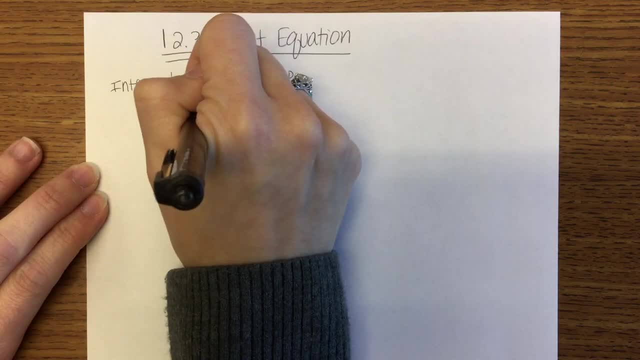 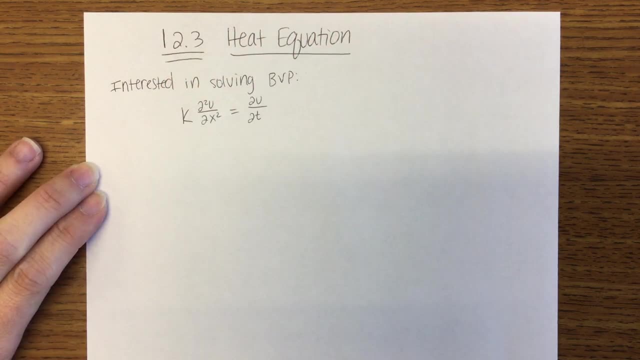 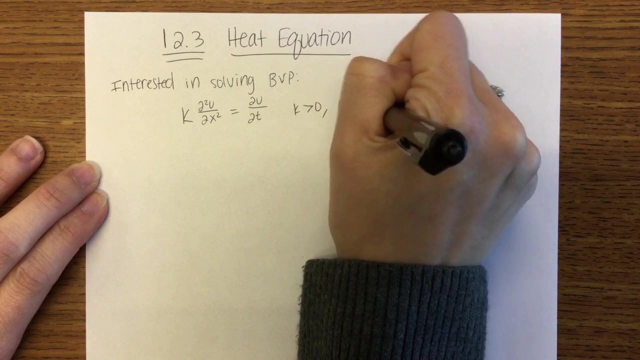 was some constant. k multiplied by the second partial of u with respect to x is equal to the partial of u with respect to t. And then a few things to remember: k is going to be positive x, which represents the spatial dimension for the rod. 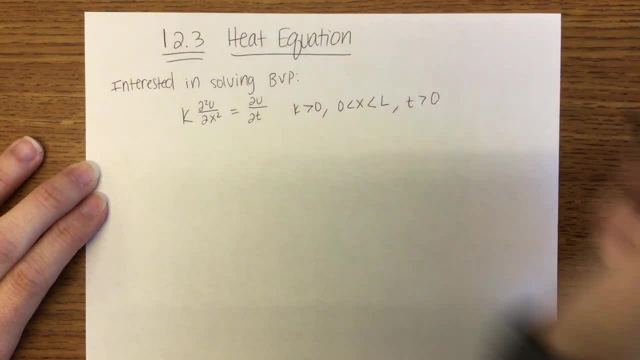 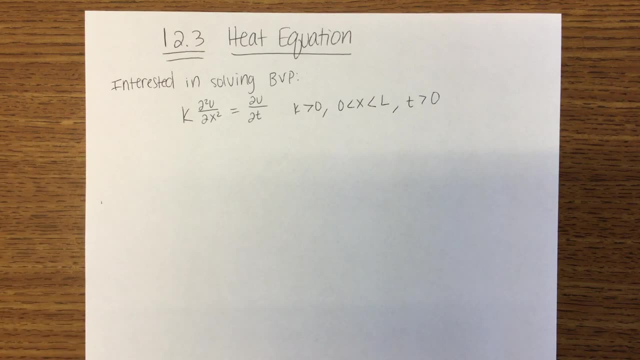 The length of the rod is going to be l, And then time is always going to be positive. Now we talked about you need to specify the boundaries, So what's happening at the end of both rods- And then you're going to need to specify the initial condition. 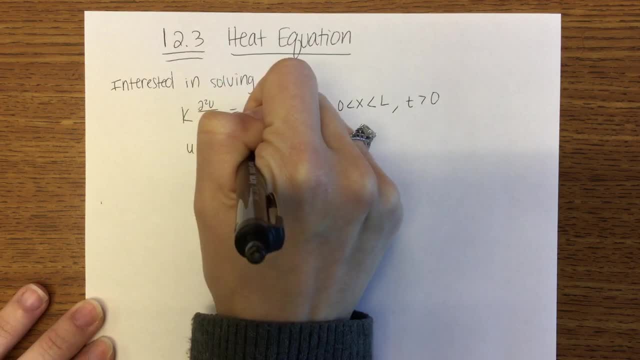 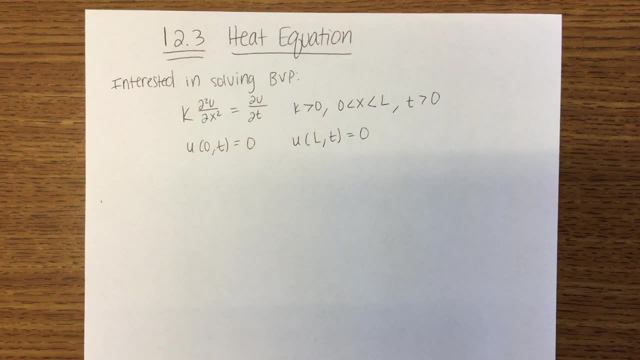 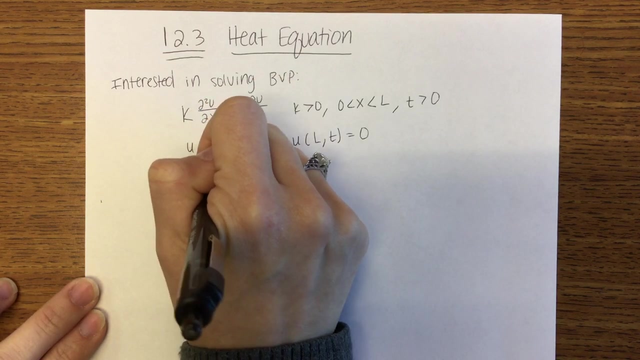 So here are our two boundary conditions: u of 0, t equals 0. And u of l- t equals 0.. What are those boundaries telling us? Temperature at both ends is held at 0.. Then we also need to specify what's happening at the beginning. 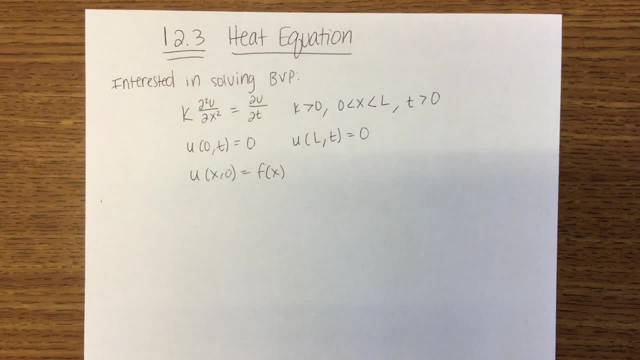 So we have u of x. 0 equals f of x. This is telling us that time 0, so the initial temperature when time is 0, is f of x. Now, sometimes you're going to know what k is, Sometimes you'll know what l is, Sometimes you're 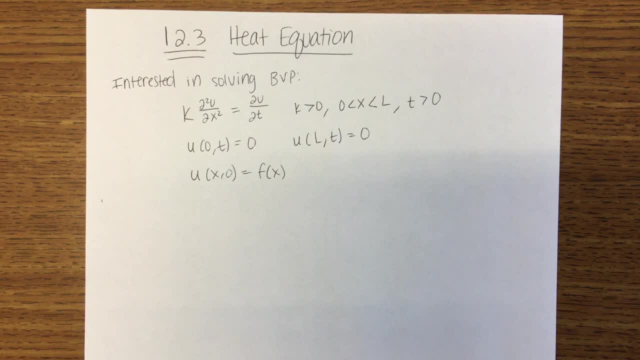 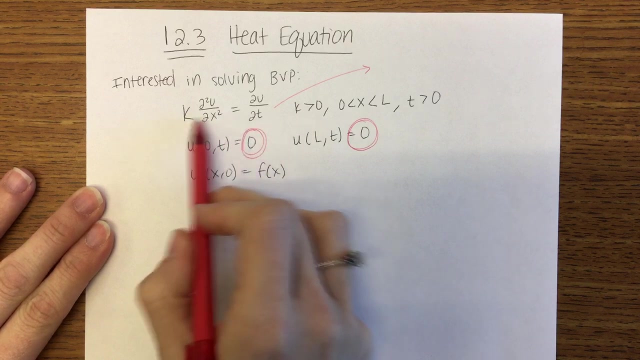 going to have a specific function for f of x. A few things to know. What makes this homogeneous is these zeros right here. So we're going to be solving with zeros right there. Another thing to know is that this notation here for the equation is pretty. 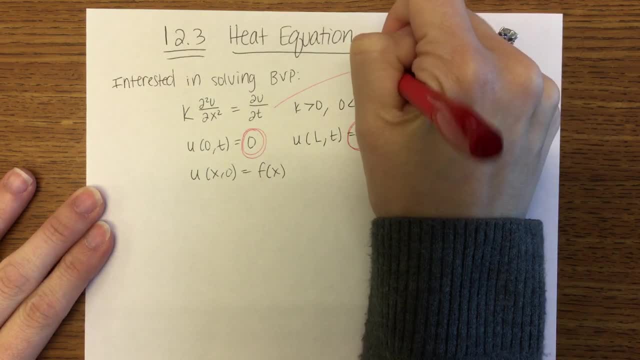 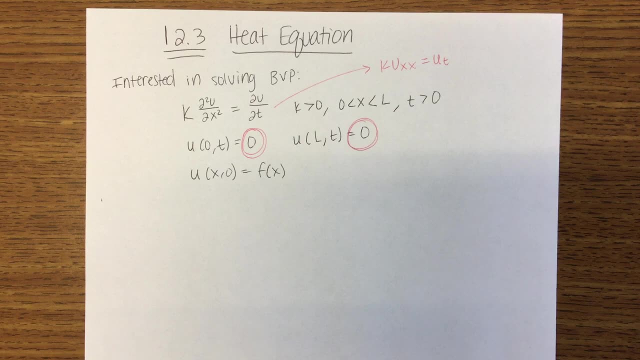 tedious, So sometimes you're also going to see the equation written like this: Same equation, just written in a different manner. Okay, so this is a partial differential equation which we've talked about is pretty complicated to solve. What is the only way we know how to solve these? 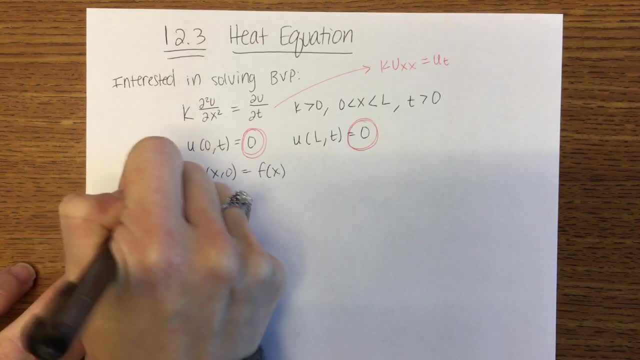 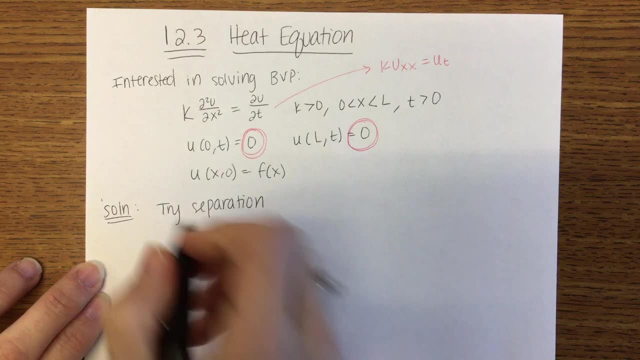 Separation. So let's try that. So we are looking for u of xt and we're going to start out by assuming that our u is the product of a function of x and a function of t, So we're going to have big x is a function of x. 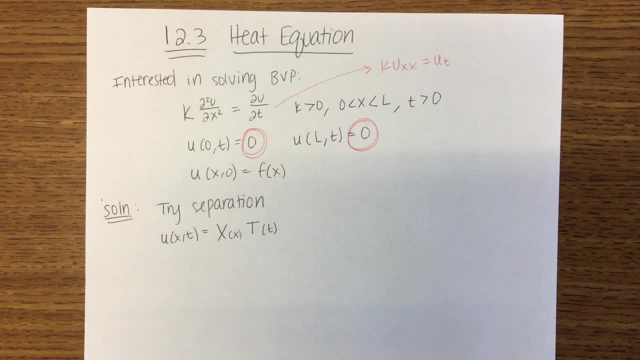 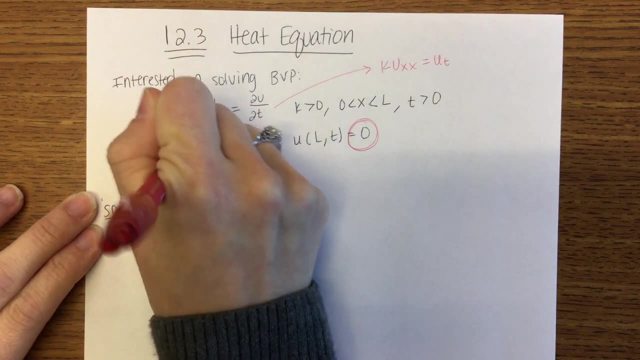 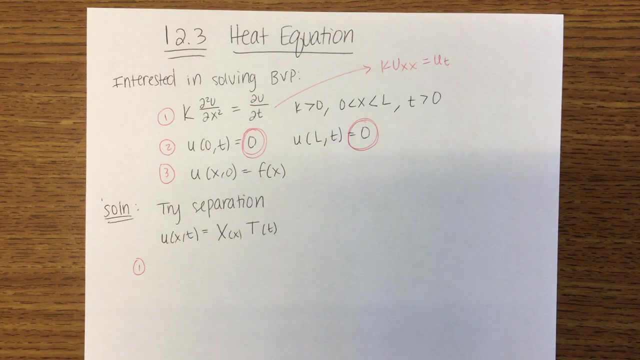 and then big t is a function of little t. I'm going to number these equations, or the equation and the conditions, because we're going to need all of those at a certain point in time. So if we use our u of xt and we plug it into this first equation here, 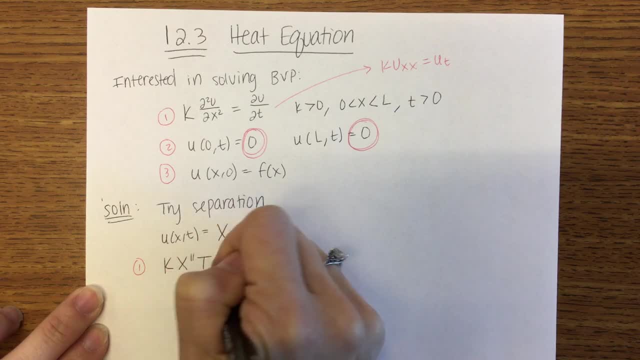 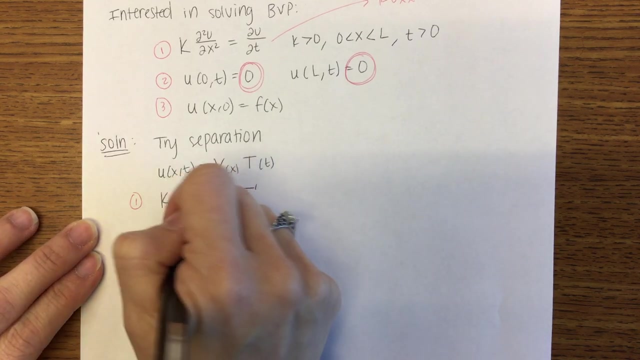 we're going to get k times x double prime. t equals xt prime. And again, remember, I'm dropping the little x, so this is not a variable x, this represents a function. So if I separate, I'm going to get x double prime over x. I'm going to move the k over to keep it. 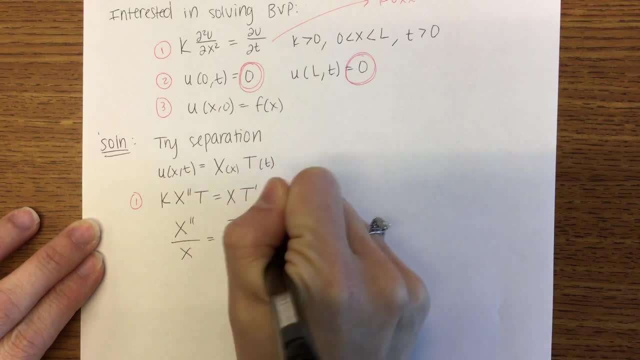 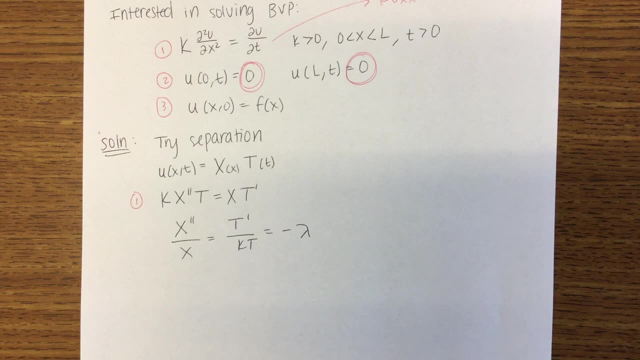 with the t, so this will be: t prime Over kt equals negative lambda. This gives us two equations, one in terms of x and one in terms of t. So the equation in terms of x is going to be: x double prime. add lambda times x equals 0.. 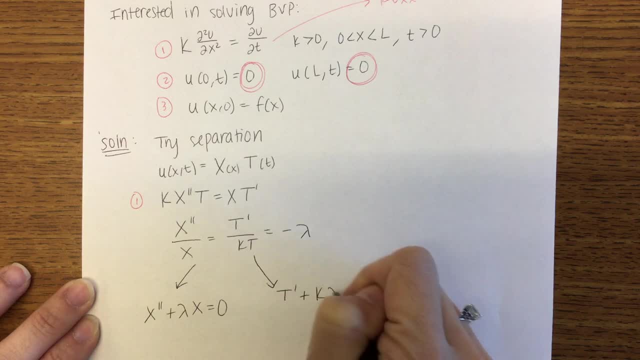 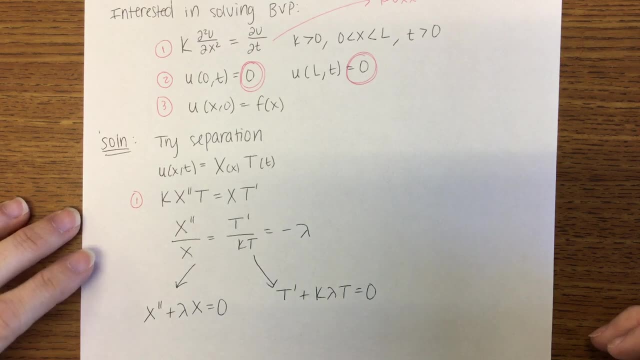 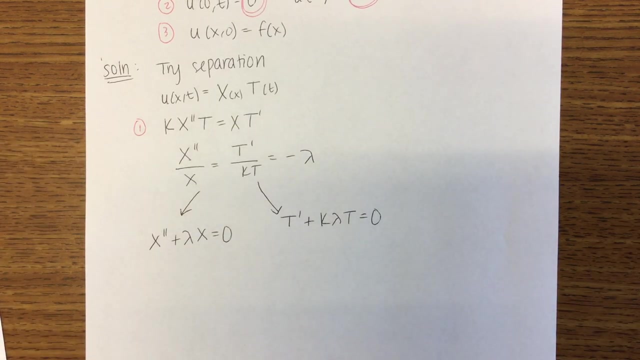 One in terms of t will be t prime. add k lambda times big, t equals 0.. Okay, For which of these equations, first one or the second one? do we need to consider all three cases? First one: Do we need to consider multiple cases here? 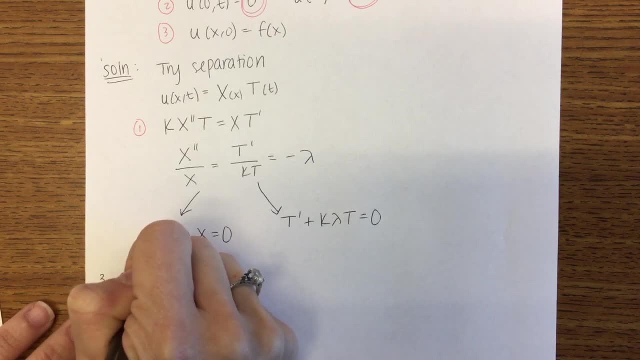 No, Okay. So we're going to start with the left equation, because it's a more complicated one, and we're going to look for the three different cases, First case being: lambda equals 0.. Now, do you guys remember going through all these various cases and solving them? 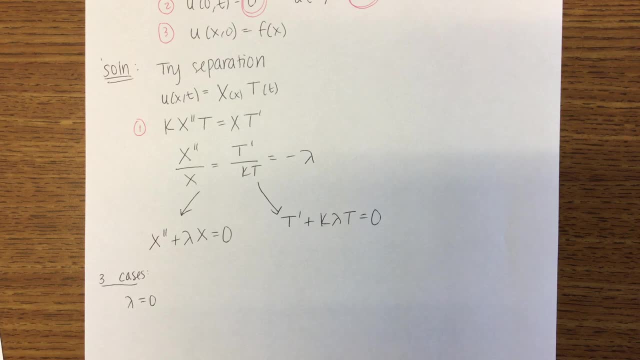 Okay, I don't want to be repetitive, so it's okay if we don't go through and solve again. Rachel, Yes, but how do you know which one has multiple cases If it has a second derivative? that's where you're going to have to consider the different cases. 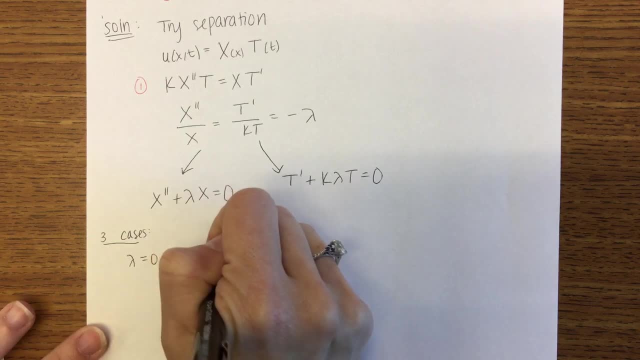 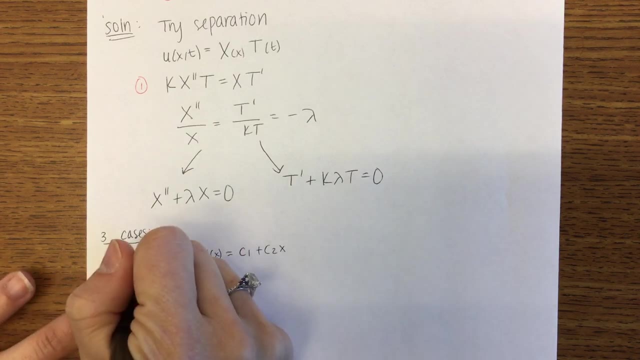 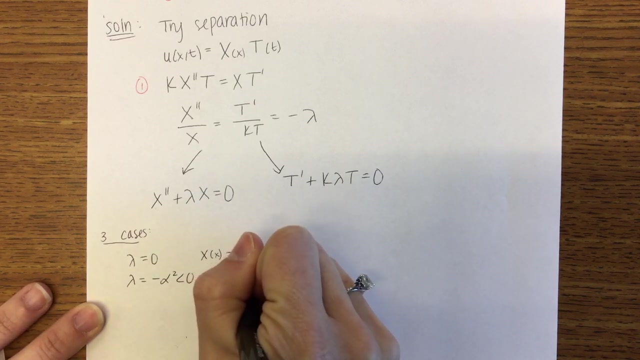 Okay. So in the case where lambda equals 0, we get big x of little. x equals c1 plus c2 little x If that lambda equals negative alpha squared. so if lambda is negative, this is negative. So in the solution we get a c1e to the negative alpha x plus c2e to the alpha x. 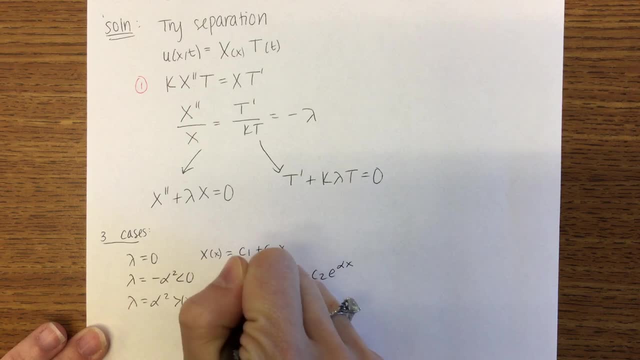 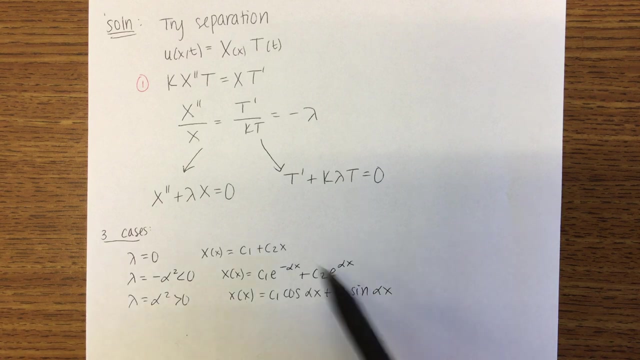 And then, in our case, where lambda is positive, we get c1 cosine alpha x plus c2 sine of alpha x. Now we are not interested in all three cases. We want to know which of these cases are going to give us non-trivial solutions. 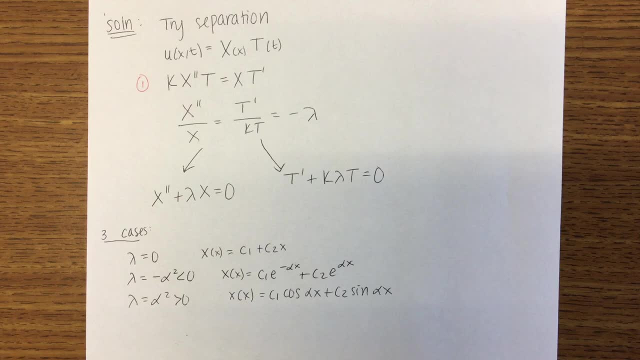 When we look at the conditions above. So far, we only looked at the main equation. We didn't look at the boundaries, which were the two conditions listed under 2.. And under 3, we didn't look at the initial value yet. 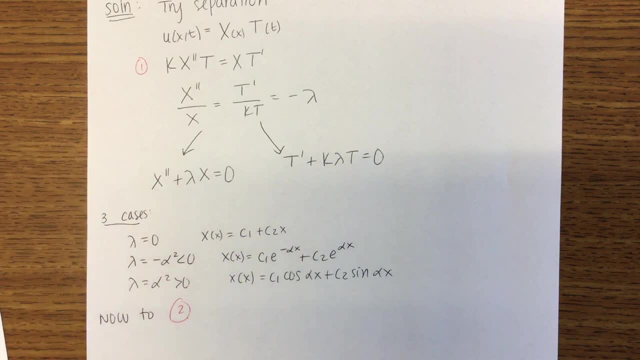 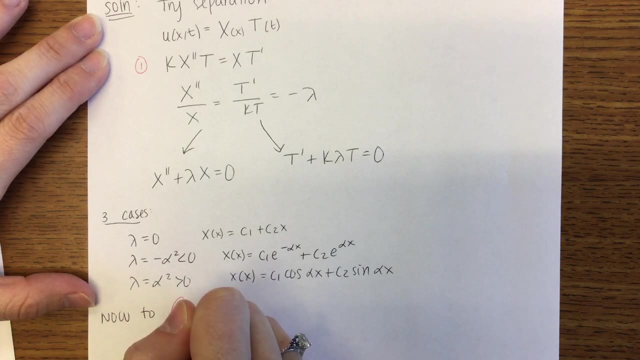 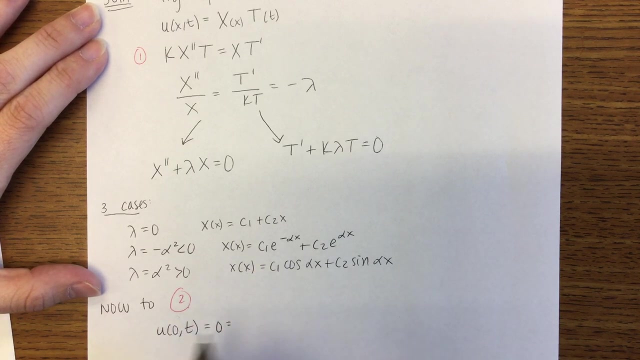 So now we are going to go to those two boundary conditions that we wrote above. So first we wrote that u of 0t is equal to 0. Now this means putting a 0 for x, So that would be x of 0 and t of t. 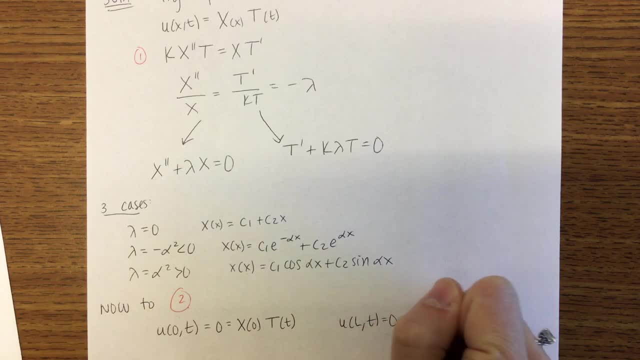 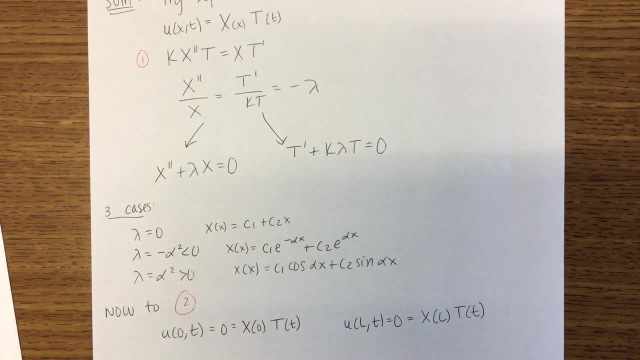 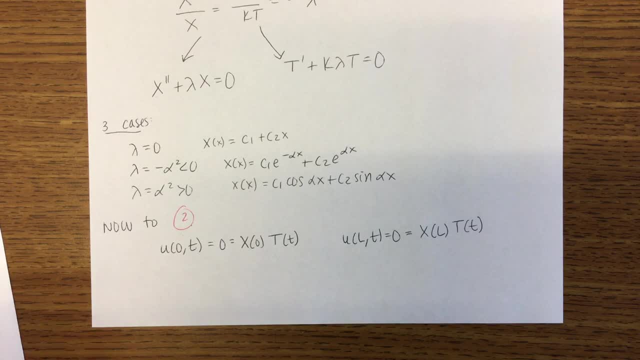 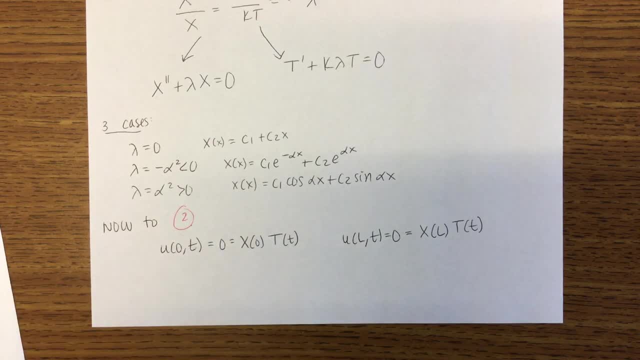 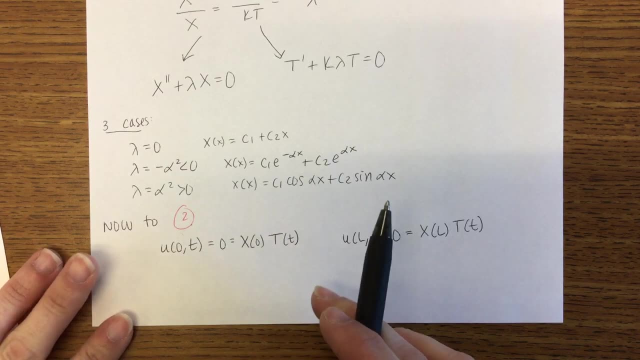 Which one do you think I'm interested in? X being 0 or t being 0?? What happens if this is 0? Trivial, Right. Then we are going to be 0 for all values of t. Okay, Okay. 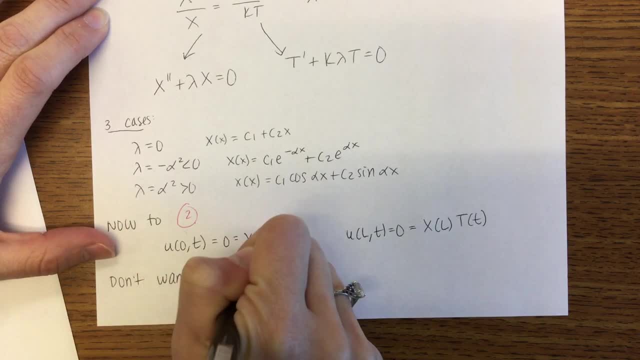 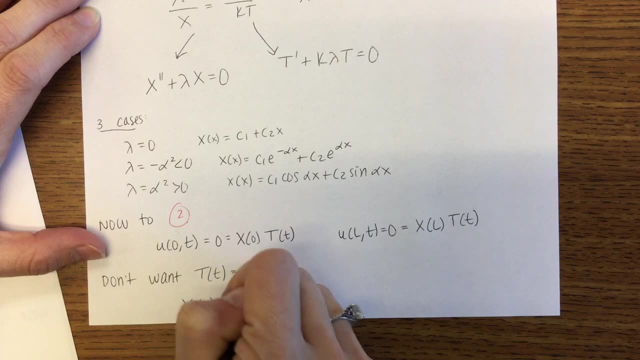 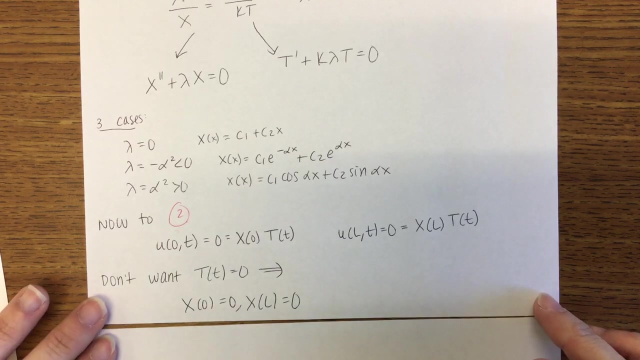 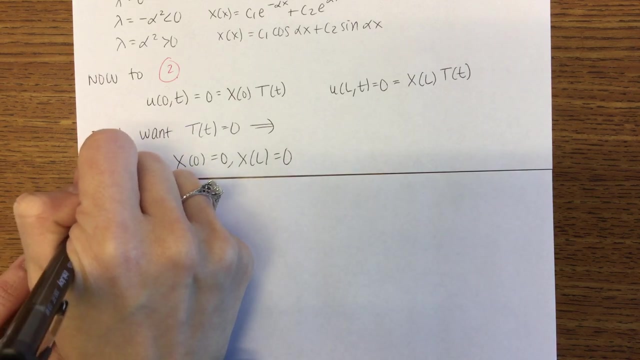 So we don't want t of t to be 0, because that would give us trivial solutions. That then tells us that x of 0 is equal to 0, and big X of L is also equal to 0.. So now we go back to the three cases. 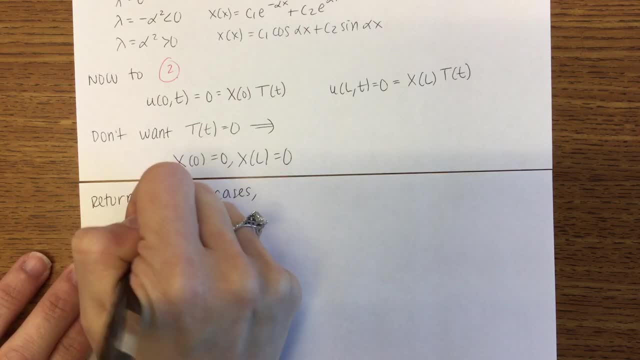 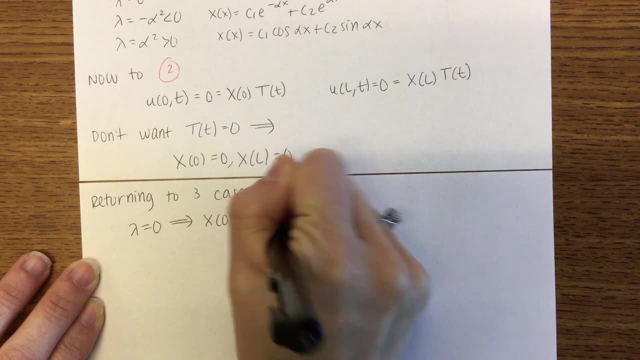 Okay, first case where lambda equals 0. If I substitute in: x of 0 equals 0, and x of L equals 0, do you guys trust that I did that correctly? Like: is it okay if we don't go through the actual substitution? 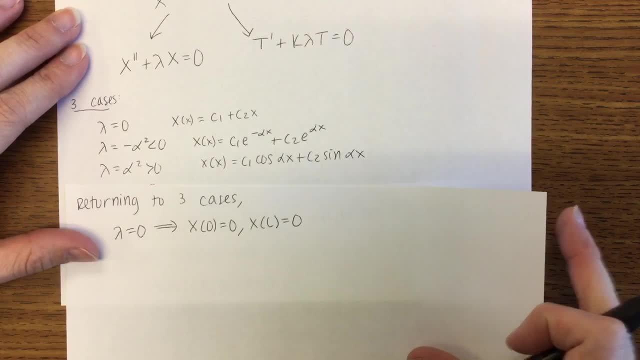 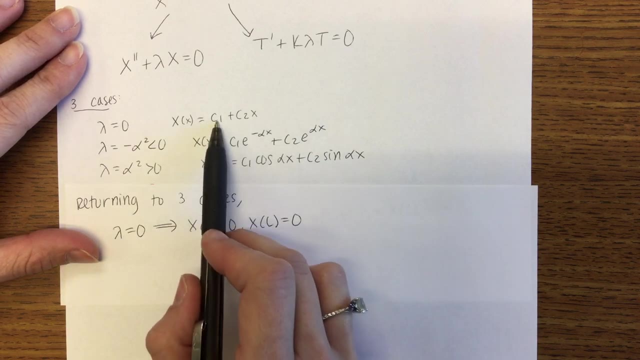 Okay, I don't think we know what I'm talking about. So if I go back here and I plug in, If I plug in 0, 0, that's going to give me a c1 of 0.. If I plug in x of L equals 0,, that's going to give me c2 equals 0.. 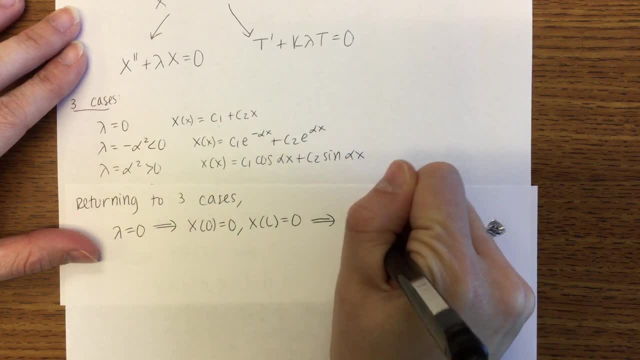 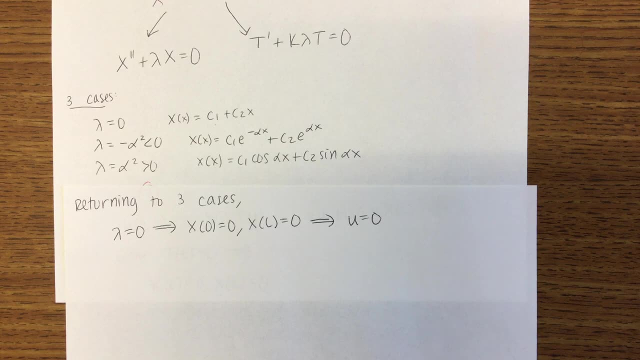 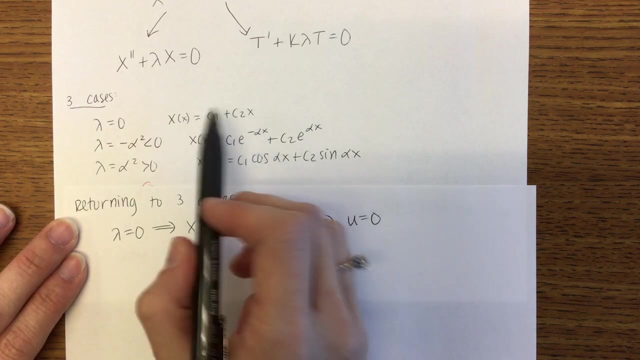 I'm going to end up with x equals 0.. So ultimately I'll end up with u equals 0.. Guys, why are we looking at me like we have no idea what I'm doing? It's a boundary value problem. Are you comfortable plugging these two points in to find c1 and c2?? 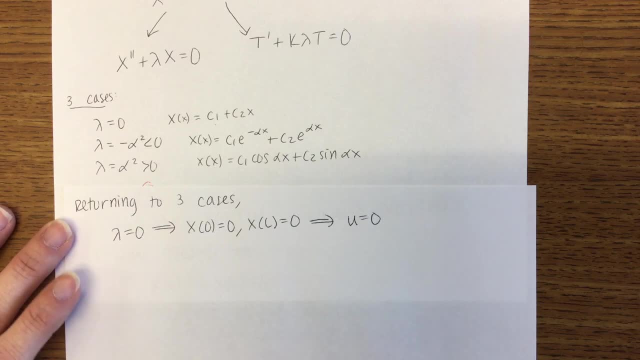 That's what I'm asking you. Okay, going with the majority here. If you're not, we'll figure it out later. Oh, you just mean like plugging in 0 for x, for little x, and plugging in 0 for 3x too? 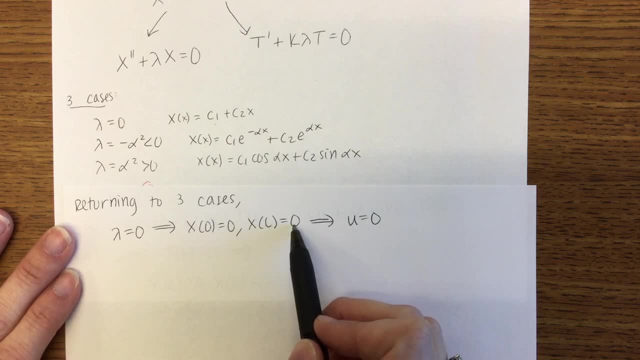 Yeah, And then in this case, this is little x, that's big X, Solving for c1 and c2.. Everybody with me now together, Okay. so we're okay if I don't actually do that for all three cases. 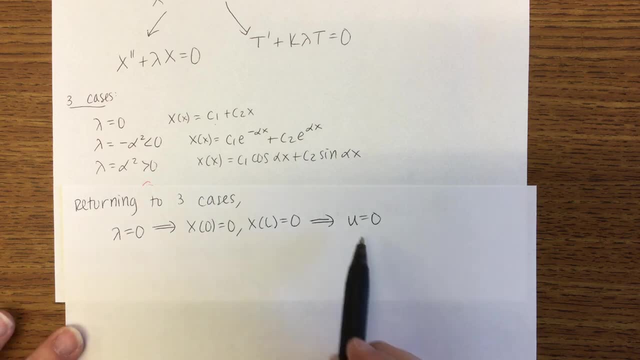 and I just show you what the result ends up being. Okay, This will always be the case. So what I'm telling you is that This case here we are not interested in, because we end up with this trivial solution- If we look at lambda- being negative. 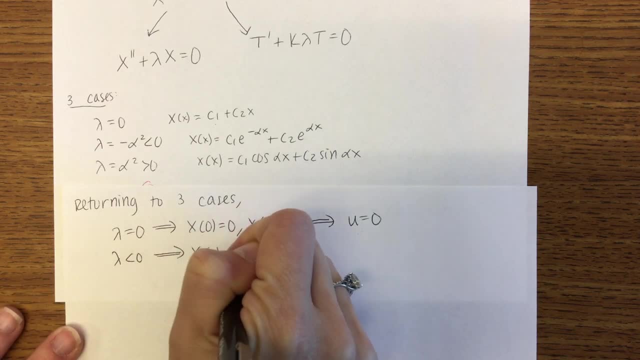 this again will give me big X of little, x equals 0, and u equals 0.. You can go through that yourself, But what this is telling us is these two cases we don't care about, We don't have to consider. 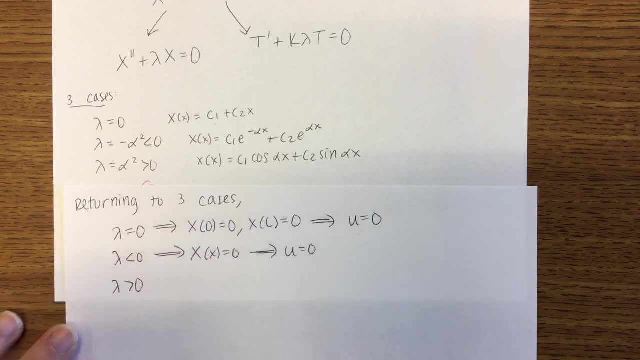 The only one that we really care about is when lambda is positive. If lambda is positive, if I plug in, X of 0 equals 0, this will be 0, this will be 0, c1 then will have to be 0. 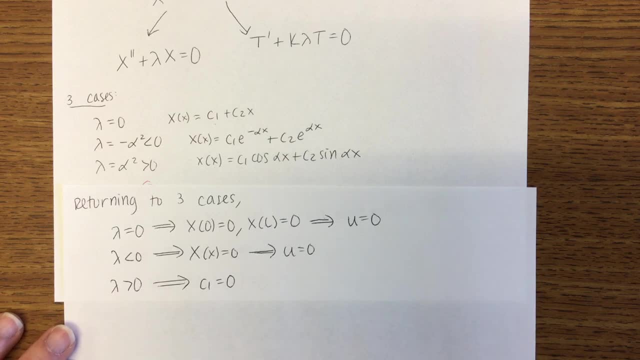 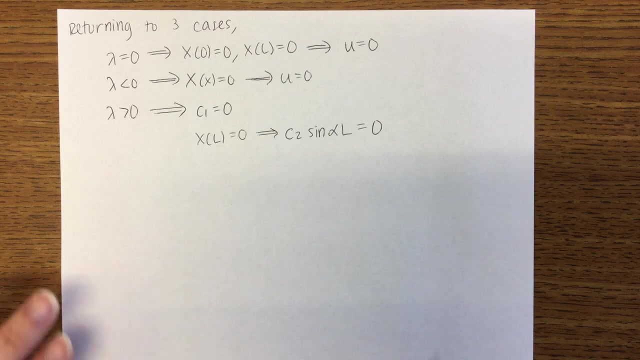 So this gives me c1 equals 0. We also know that X of L equals 0. So that will be c2 sine of alpha. So that will be c1 times L has to equal 0.. Okay Then, do you guys remember doing this before? 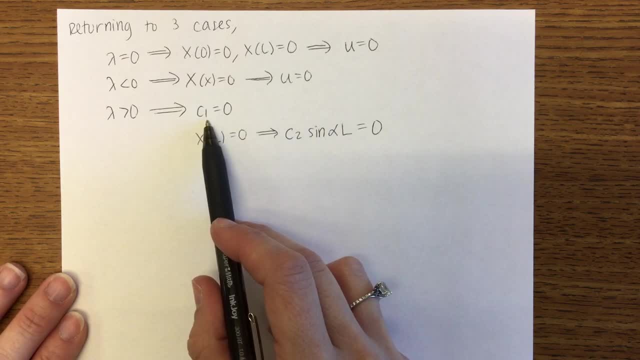 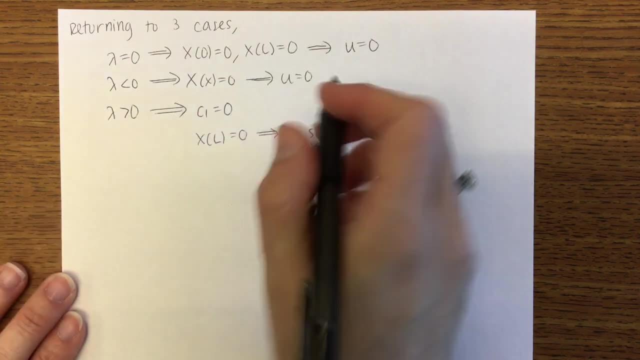 We said we don't want c2 to be 0, because we already got c1 to be 0. That will be trivial. So then we said we really want this sine to be 0. So we said that sine is 0 at n times pi. 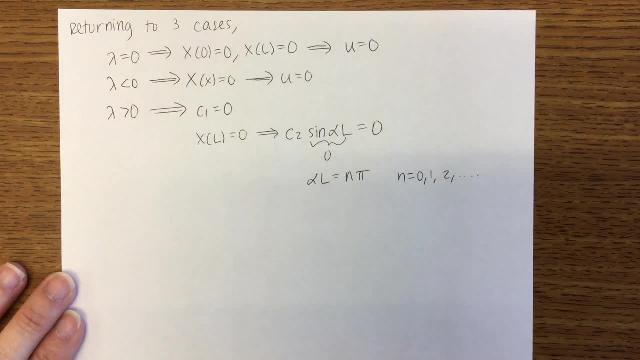 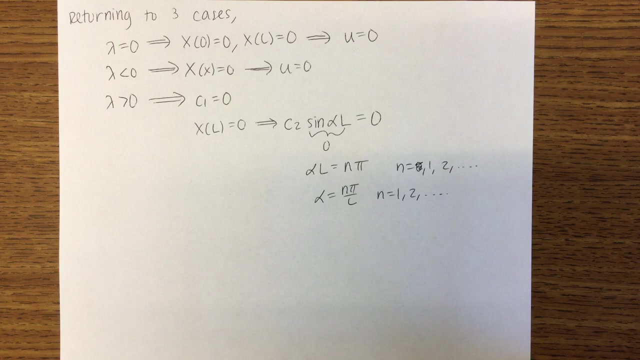 If n is any integer. So we got our alpha to be n pi over L When n is 1,, 2, etc. Does that look familiar? Yeah, Okay, Good It should. So here's what that tells us. 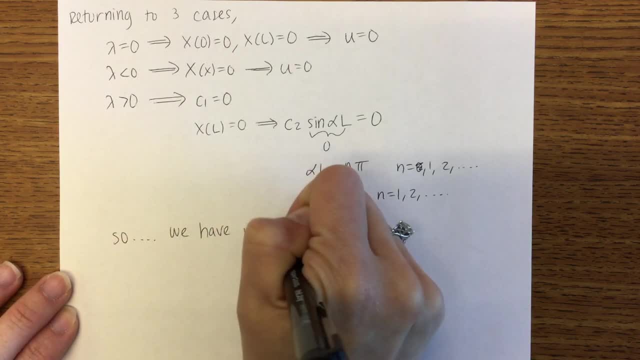 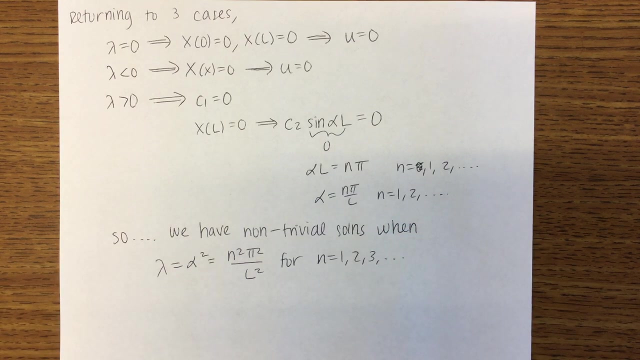 We have non-trivial solutions When that lambda, which again is alpha squared, is going to be n squared, pi squared over L squared For n is 1,, 2,, 3, etc. Why did I start n at 1 and not at 0?? 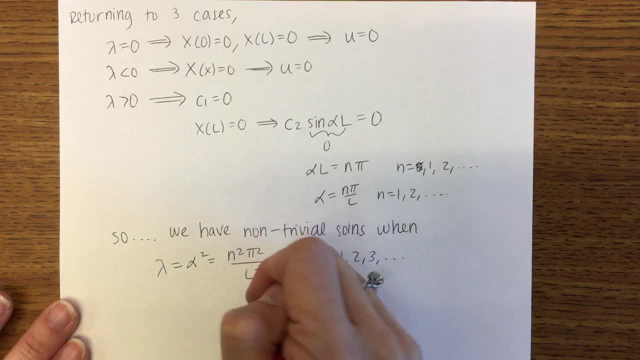 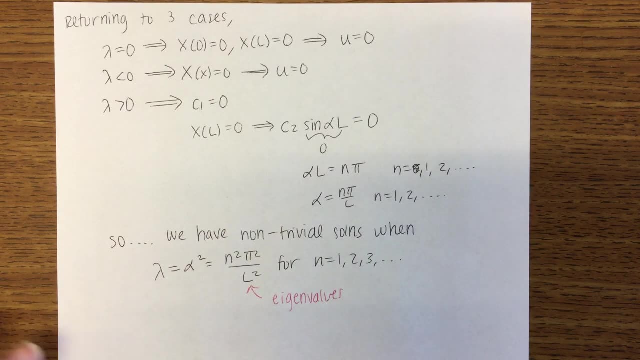 We don't want lambda equals 0. We already showed that that's going to give us a trivial solution. These were called the eigenvalues before. We then would plug the eigenvalue into the function, which in this case is big X, to get our eigenfunctions. 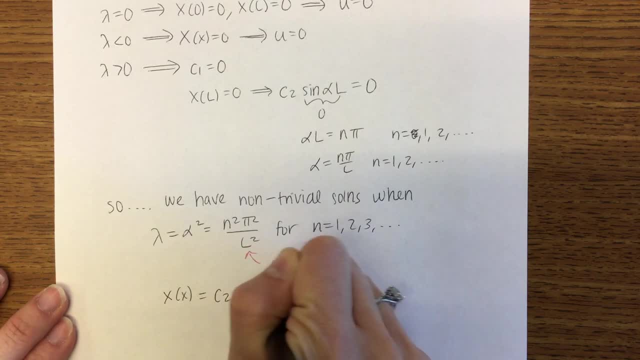 So big X will be c2, sine of n, pi over L, X Again, when n is 1,, 2,, 3. Because we have sine of alpha times, L, Okay. Okay, Now we have to solve the T equation. 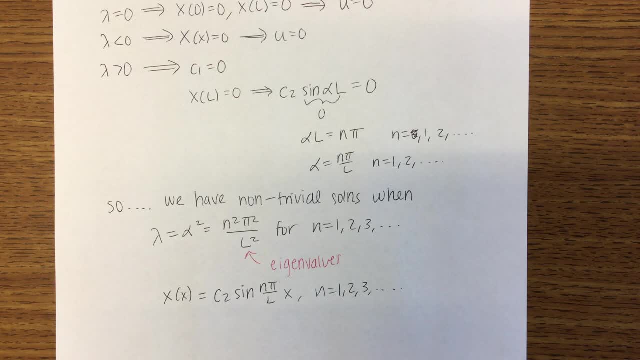 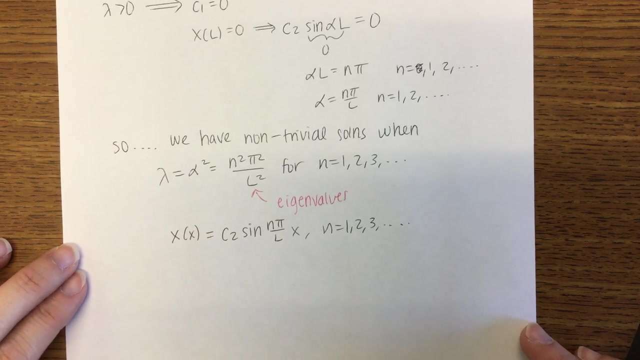 So we solved the X one. Now we're on to T. Not all I'm going to show you later. This process is yes, Yes, the process is going to work, Okay. So now we've got to go back to our second equation. 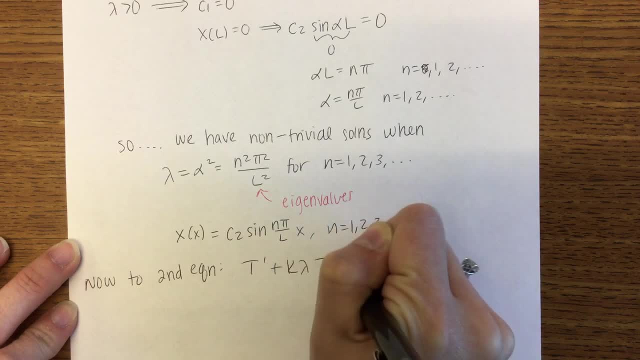 That was the T prime plus K lambda Times big T equals 0. So this is separable. You're going to get T on one side, get everything else on the other side. When you do that, you get T prime over. big T equals negative K times lambda. 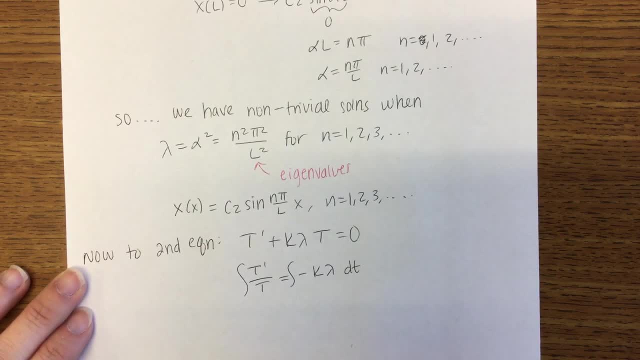 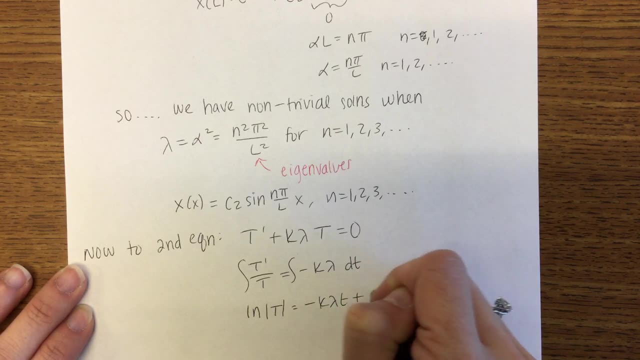 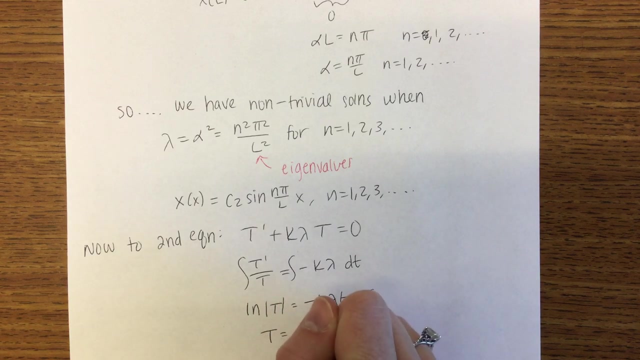 Integrating with respect to T To little t. that is So we get natural log of big T equals negative K, lambda little t plus C. Applying E to everything, we get big T is C3E to the negative K, lambda T. 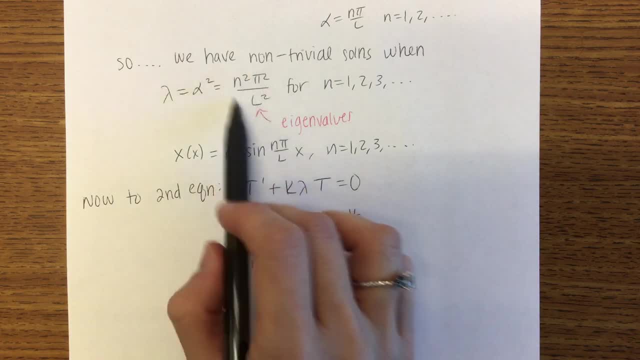 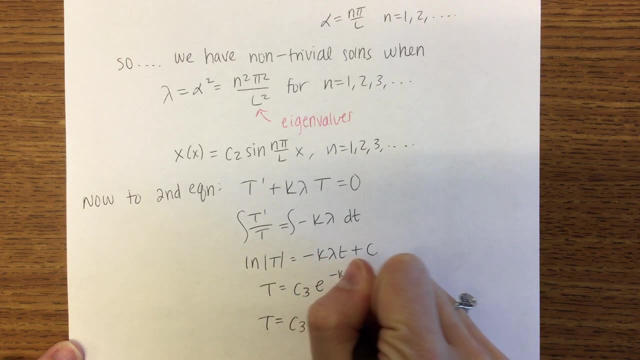 Now we know what lambda is. We know what the eigenvalue is That was defined up above. So ultimately, we get T to be C3E to the negative K, n squared pi squared over L squared times T. So that's what we're going to do. 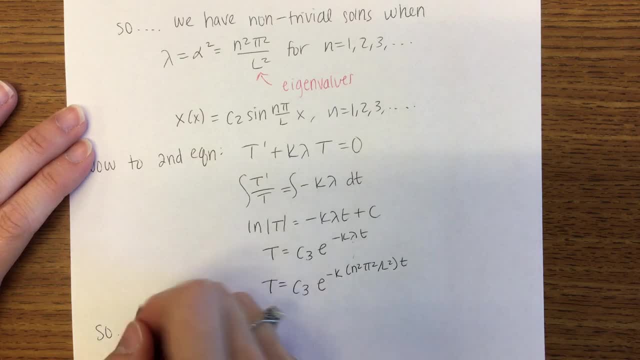 So here's where we are now: U of n, because u is going to be based on what n is, which was big X times big. T is going to be that function multiplied by that one, Multiplying those two together. I'm going to call that A of n. 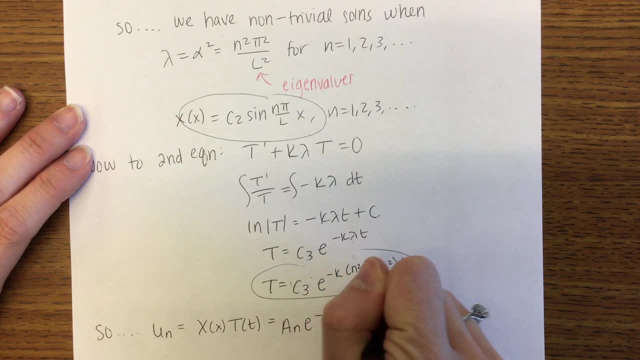 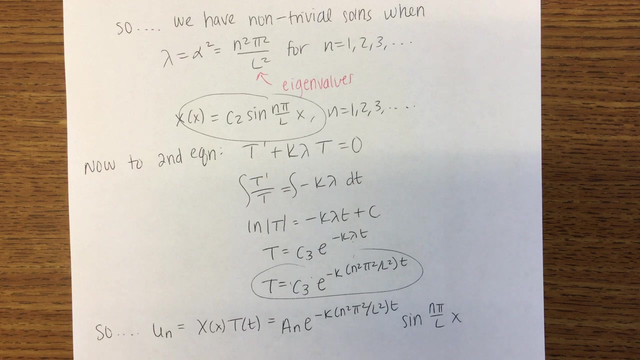 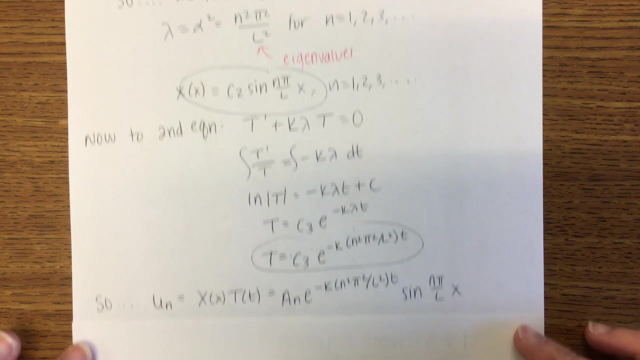 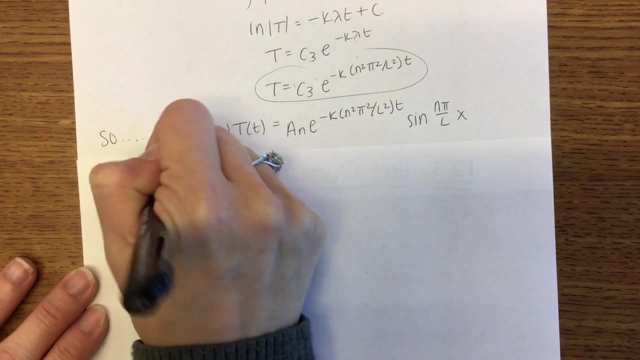 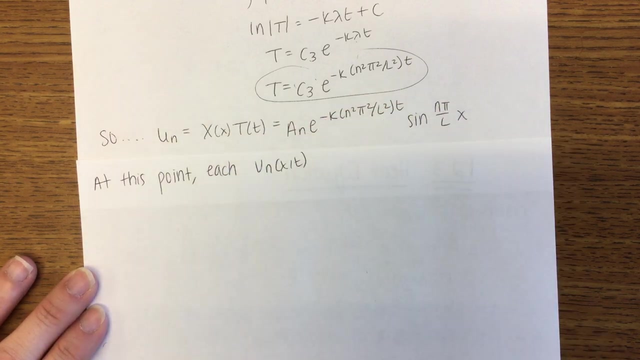 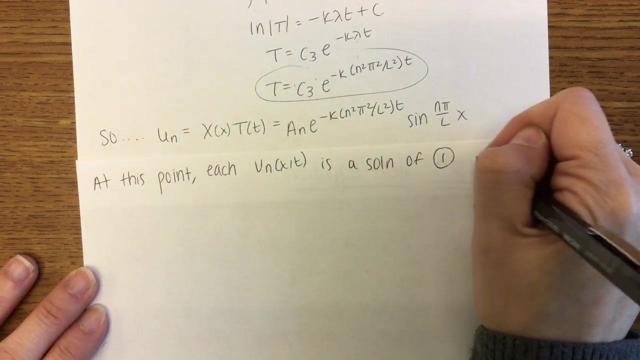 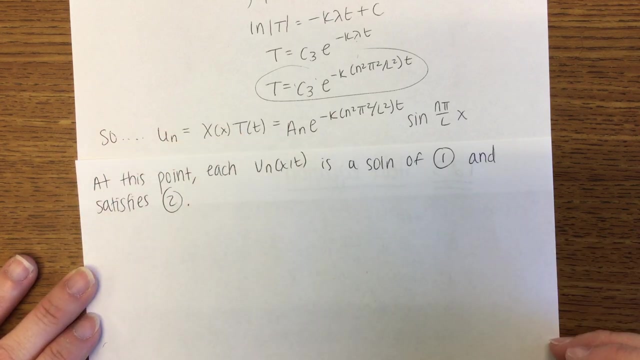 And then we have E to the negative, K n squared pi squared over L squared T, sine of n, pi over LX. Okay, Questions before we keep going. Okay, so at this point, each u? n of X, T. so what we wrote above is a solution of equation 1 and satisfies those boundary value conditions in 2.. 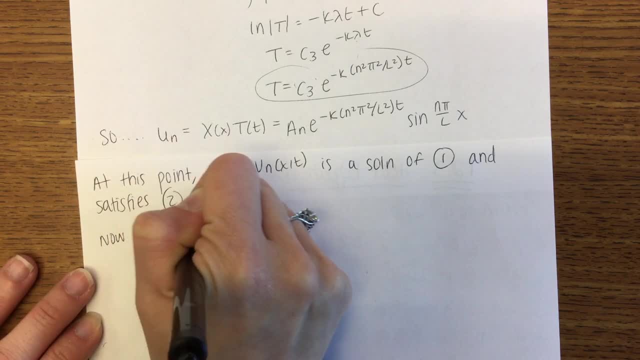 Last thing we need to consider is condition 3.. Condition 3 was that u of X 0 equals f of X. So what we're going to do is we're going to plug 0 in for T up here. When we do that, this whole exponent becomes 0. 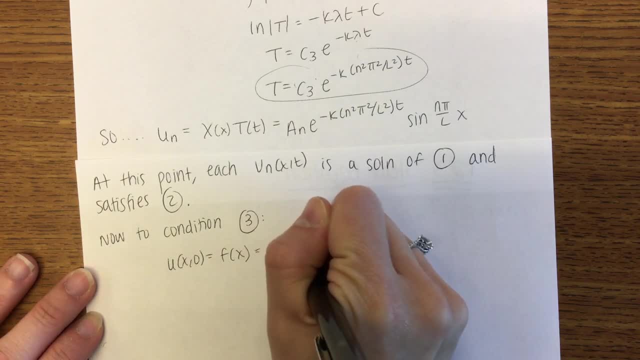 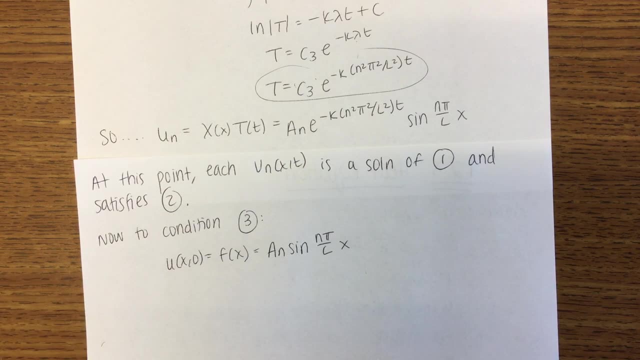 E to the 0 is 1.. So we're left with A n sine of n pi over L squared, And we're left with it plus 1 over L X. Okay, So we're not going to be able to find some reasonable f of X to give us this. 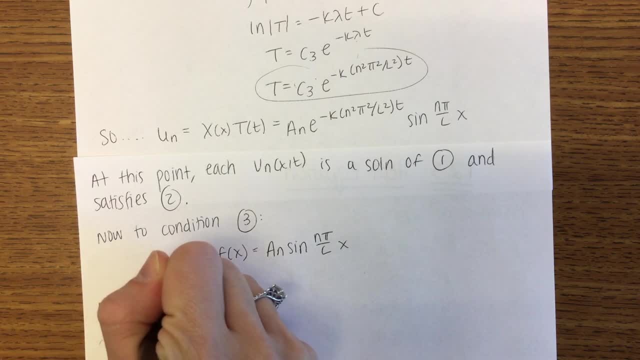 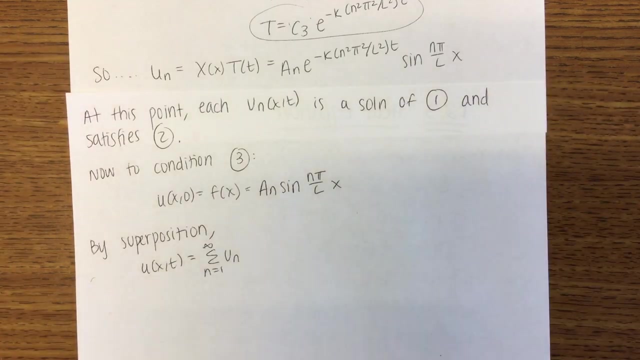 So what we're going to do instead is we're going to use superposition. So, by superposition, u of xt will be the sum from n equals 1 to infinity of u of n. In this case, that'll be the sum from n equals 1 to infinity of a of n, e the whole thing we wrote above. 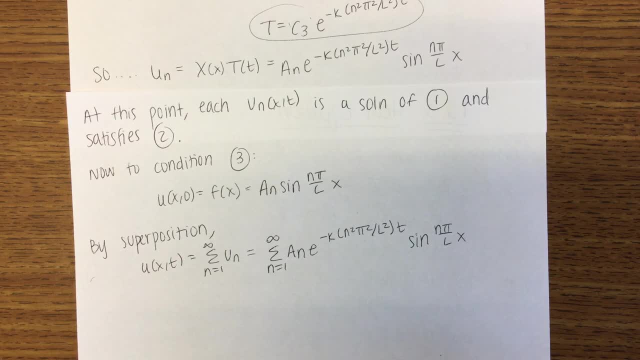 So how that helps us is if we look at u of x0 now in a similar manner, by changing n from 1 to infinity, we get that f of x to be the sum from n equals 1 to infinity of a, of n, sine, of n pi over l x. 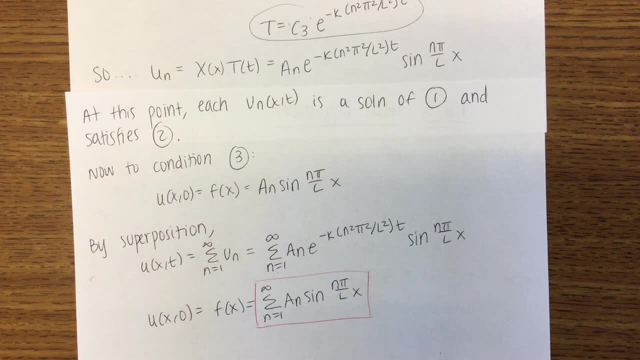 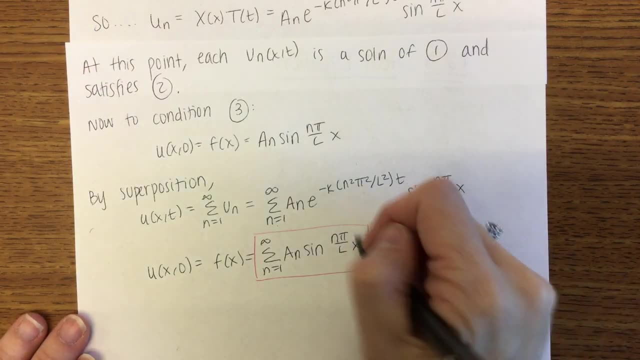 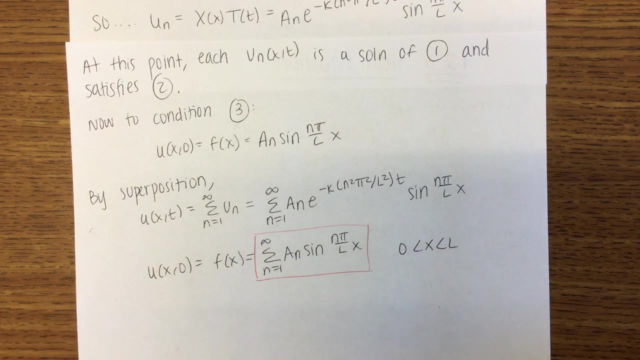 This should look familiar. We also know that x is between 0 and l. Any guesses at all? Where did we see summations like this that involved sines and cosines Foyer? Now, when we started out foyer, did we go from 0 to l? 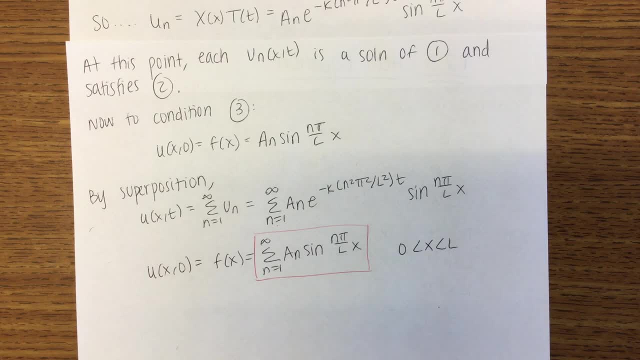 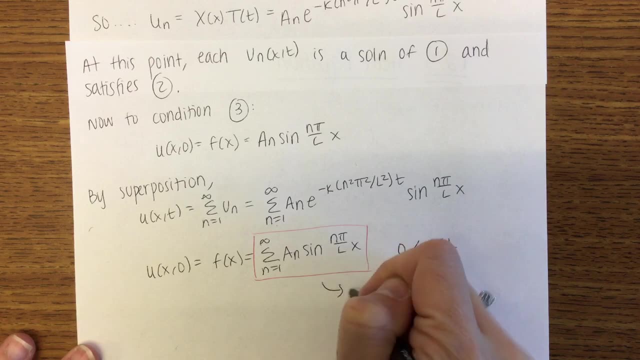 We went from negative l to l. What did we call it when we went from 0 to l? Half-range expansion. Yes, So this is a half-range expansion in a sine series. Okay, Okay, Okay, Okay Okay. 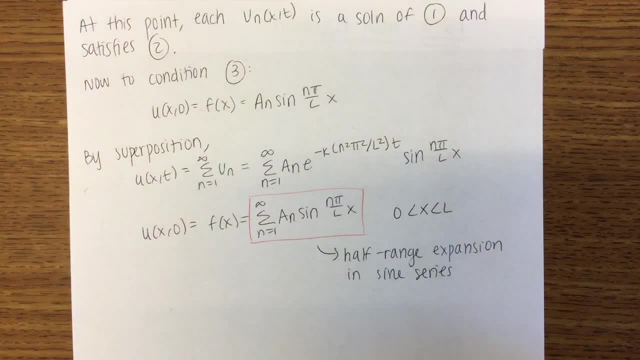 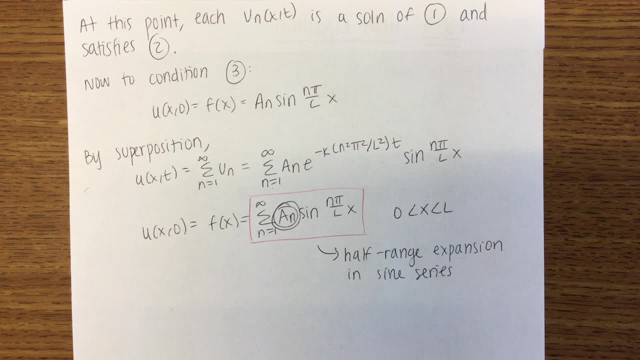 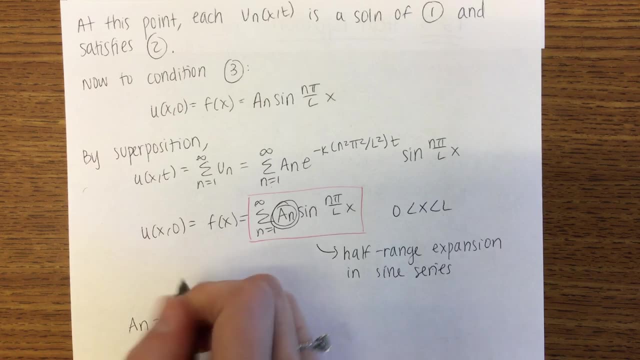 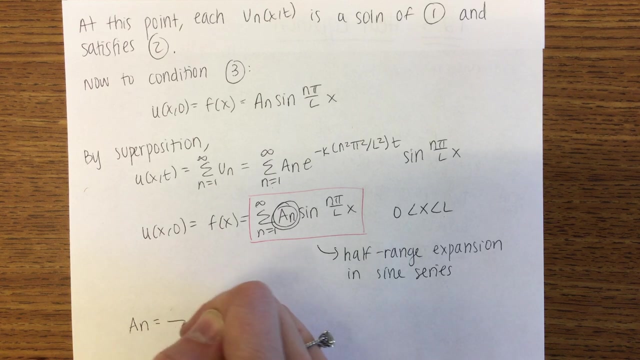 No, In a half-range expansion for sine. So I could just give us the formula: We good with that. You think you remember? Yeah, Okay, Do you remember what the coefficient out in front is: 1 over p or 2 over 2 over p? 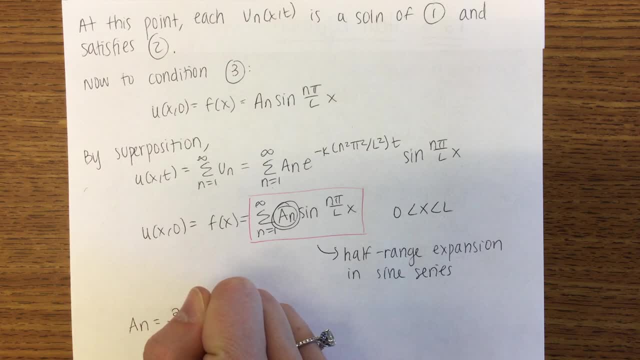 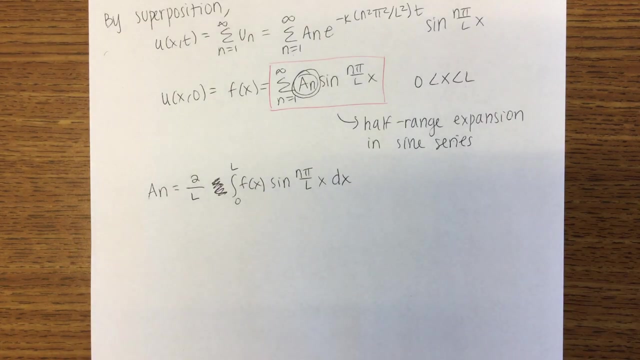 It is, In this case, 2 over l. Wow, Wow, Yeah over L. and then L to 0 of f of x, sine n pi over p or n pi over L of x. Yeah, Beautiful, Okay. so remember how you guys were like: when are we going to use this? 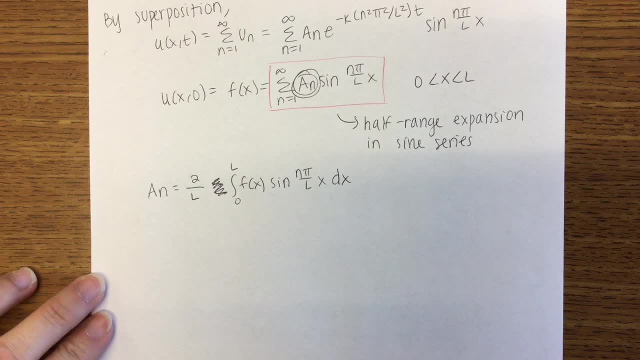 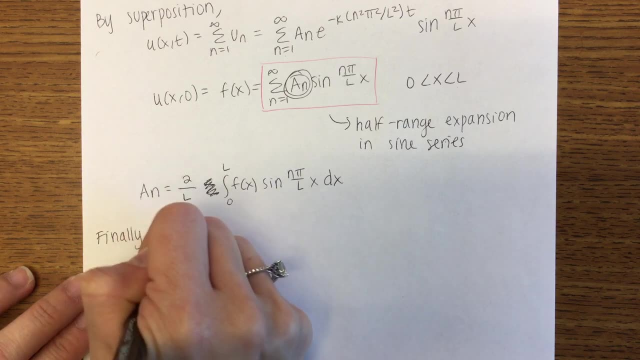 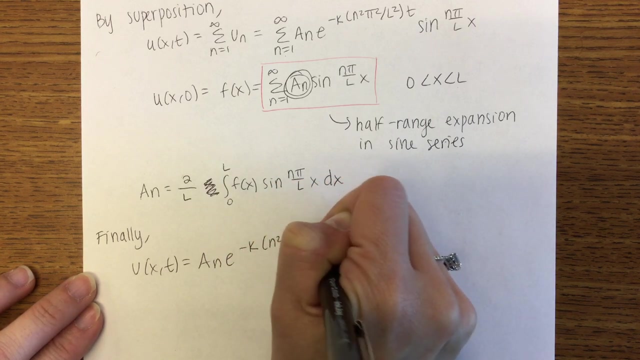 Right now. Okay, we're almost done with this one. Finally, before we had u of x, t is a of n e to the negative k, n squared pi squared over L squared t sine of n pi over L x. That's what we had before. 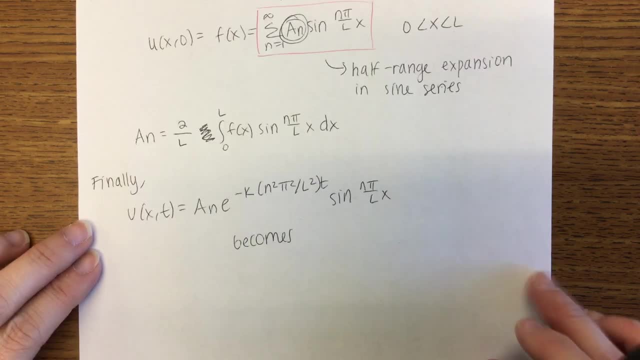 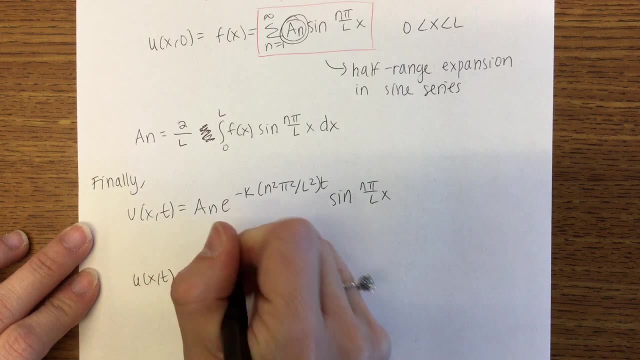 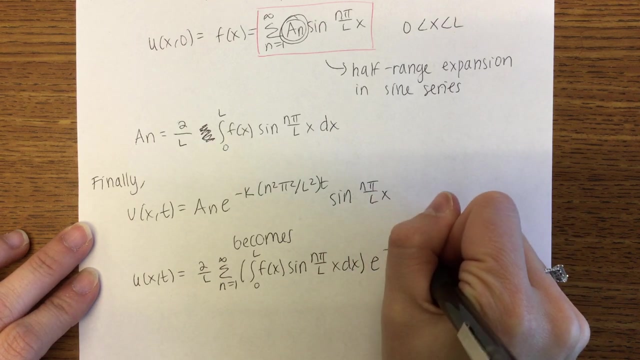 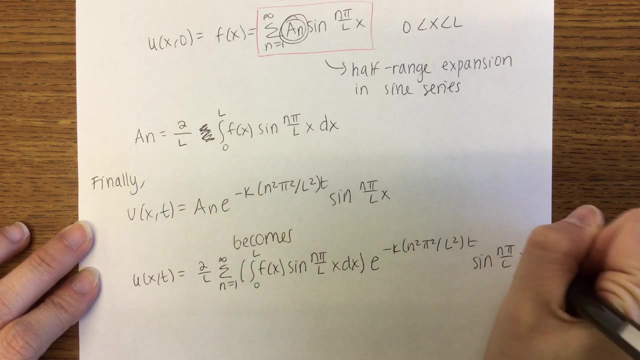 This now becomes, now that we know an expression for a of n. this becomes 2 over L. summation from n equals 1 to infinity. integral 0 to L of f of x. sine of n. pi over L x. dx, e to the negative. k. n squared pi squared over L squared t. sine of n pi over L x. 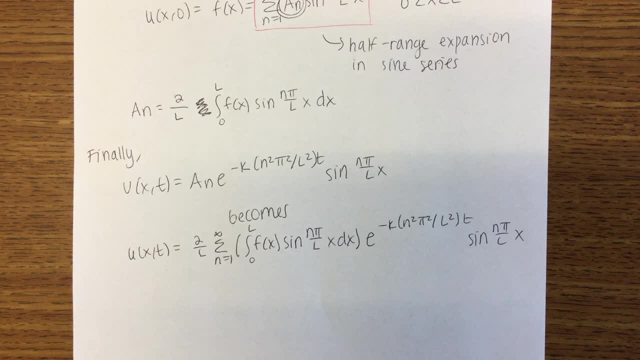 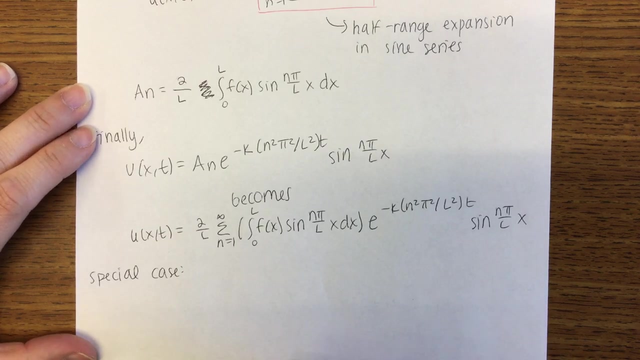 Woo, Yeah, that's the answer, I know, Okay, there is a special case of. this Special case is the case where u of x 0 equals 100.. So the initial temperature throughout is 100.. L- L is equal to pi. 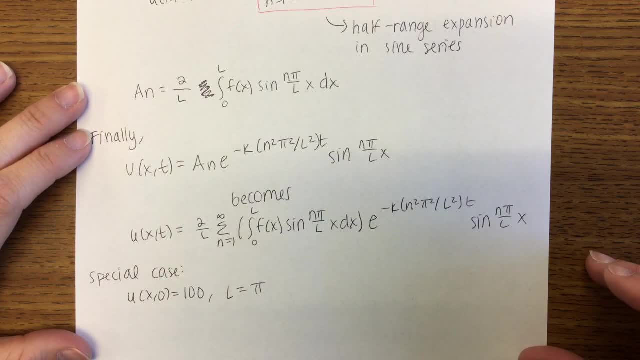 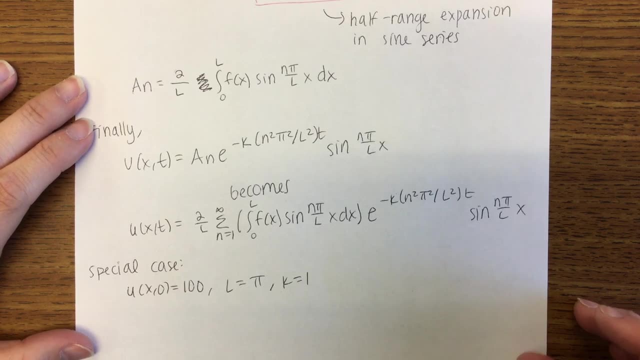 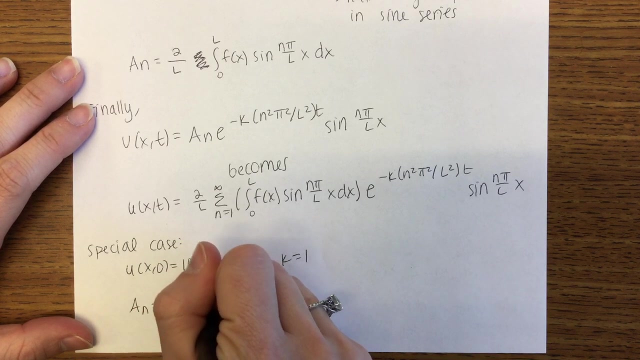 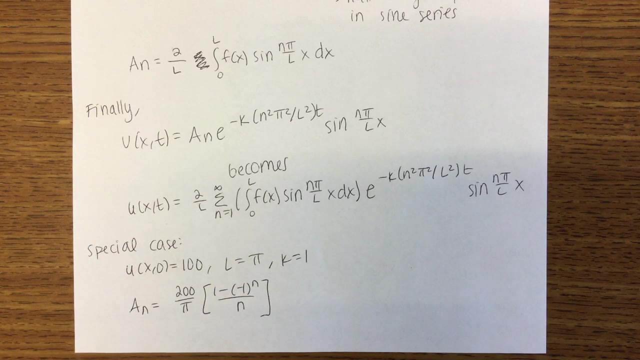 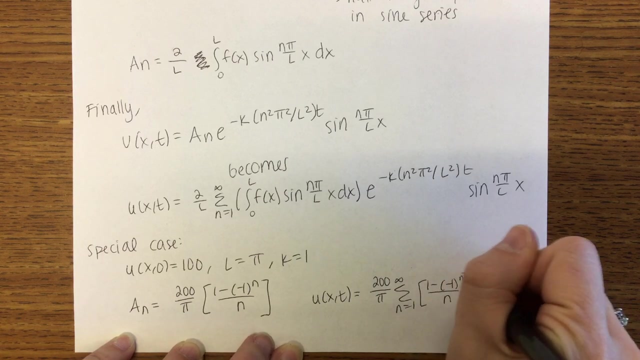 What is that telling us? The length of the rod is pi, And then k is 1.. If that's the case, a of n becomes 200 over pi, 1 minus negative, 1 to the n over n, And hence u of x, t is going to be 200 over pi. the sum from n equals 1 to infinity of that, 1 minus negative, 1 to the n over n, e to the negative n squared t, sine of n- x. 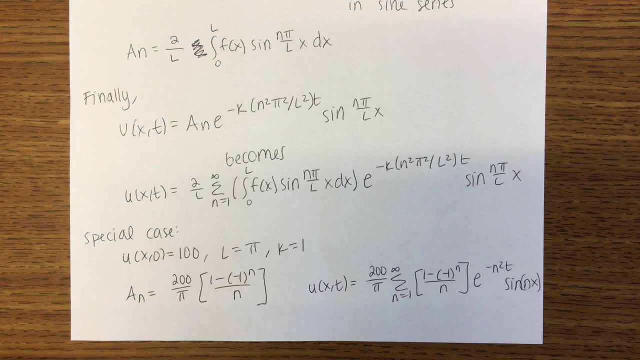 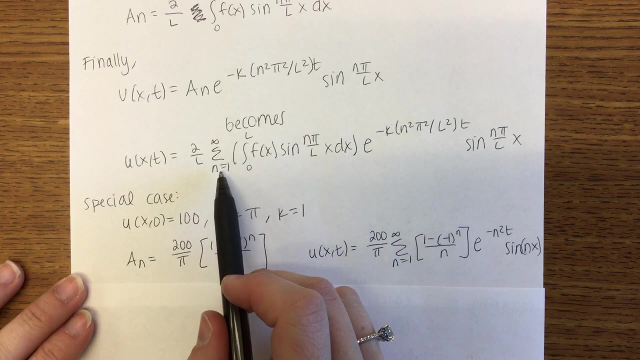 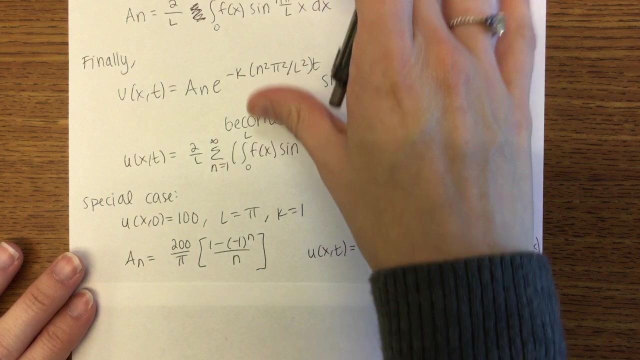 Thanks, Yes, We wrote finally the first one underneath that Should there be the summation sign above the next one in front of a n. Should there be a summation sign there? No, Then where does it come from? So this: 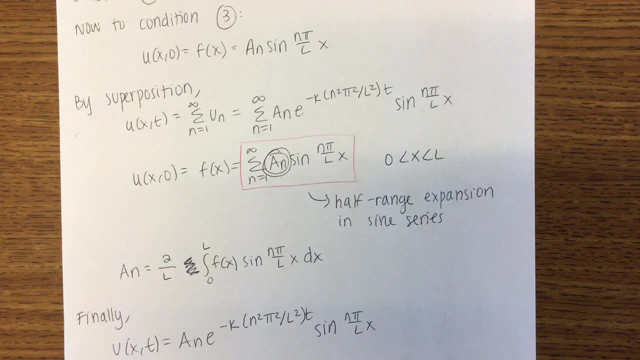 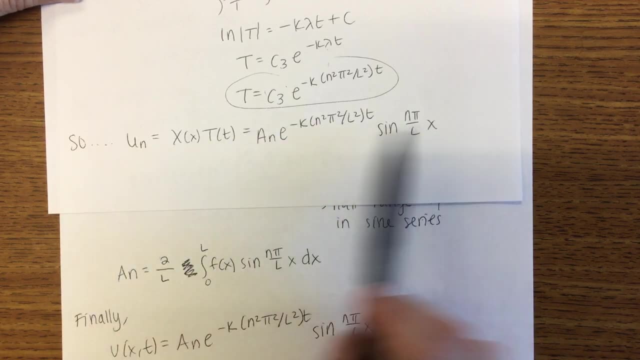 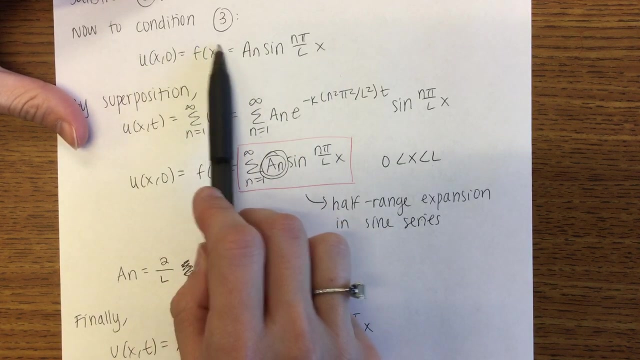 This is where we were before, right here: Uh-huh, Yeah, Yeah, Yeah, Yeah. And then we said we need to find some expression for a of n. So that's when we looked at this condition and we said we're not going to be able to find an f of x. 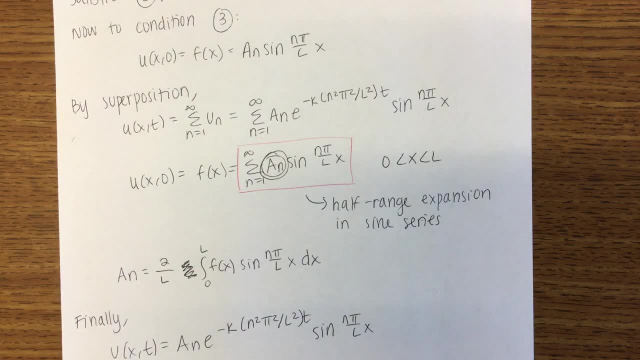 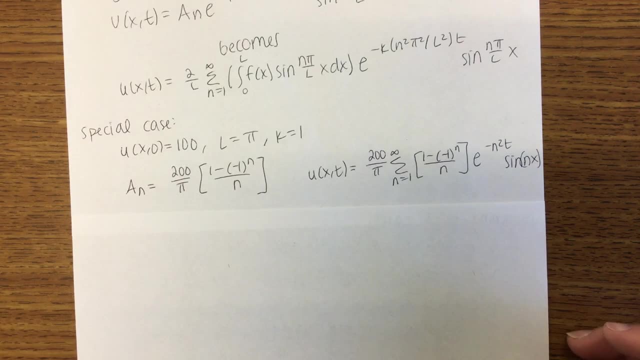 Okay, Okay, Is that enough? Yeah, Okay, You guys ready to see what an example of this actually looks like? Yeah, Good, I'm excited For those of you who like to plan. we have one and a half more pages. 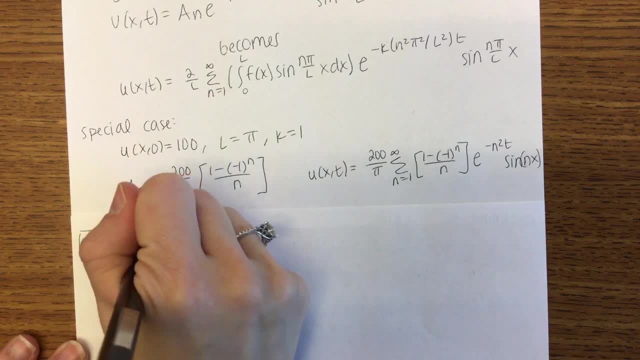 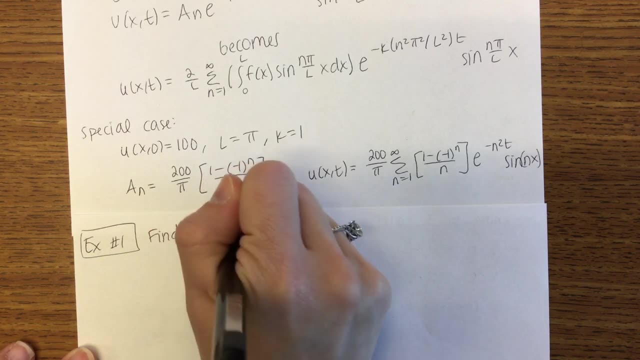 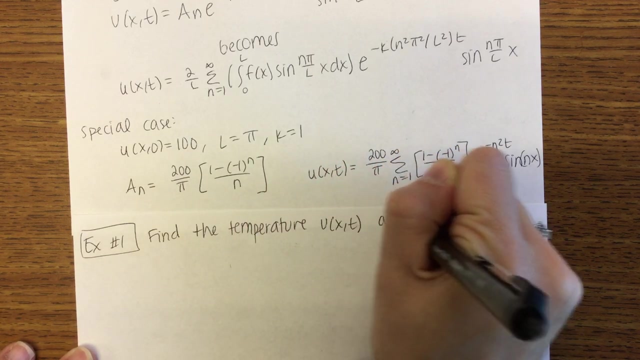 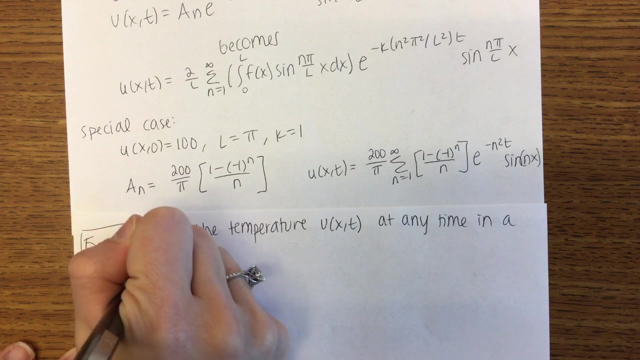 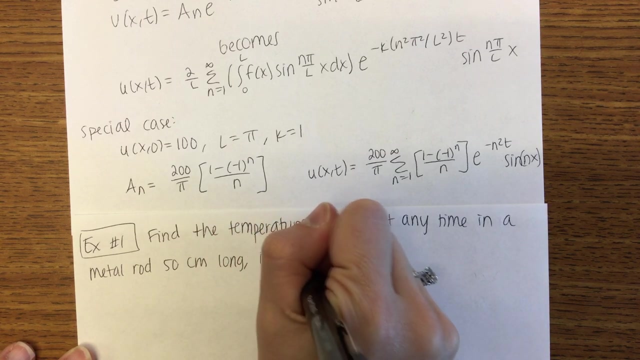 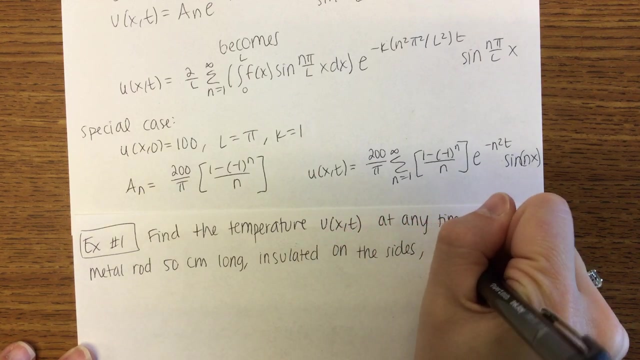 Of notes. My guess would be No. Oh, I guess we'll see. Okay, Find the temperature U of xt at any time In a metal rod 50 centimeters long, Insulated on the sides Which initially 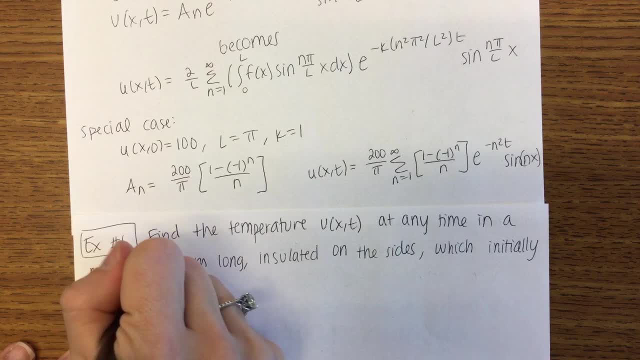 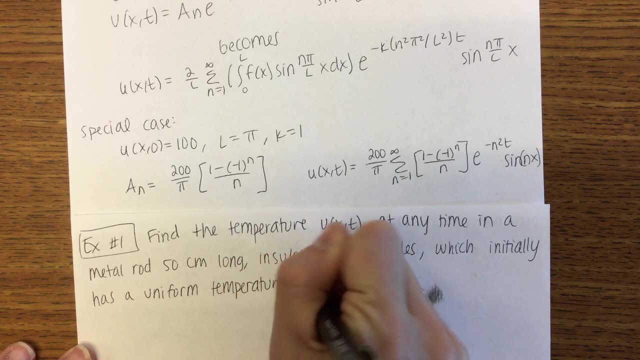 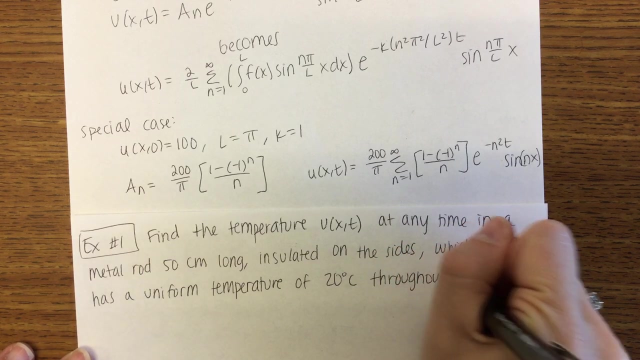 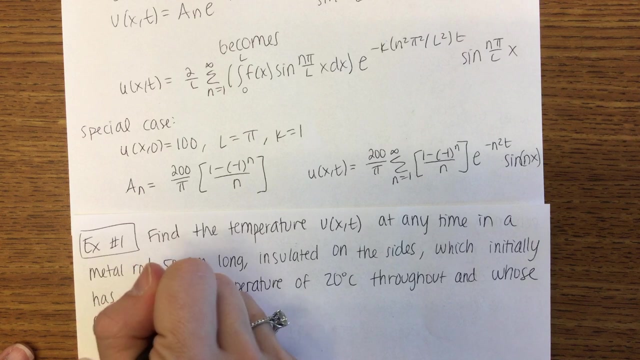 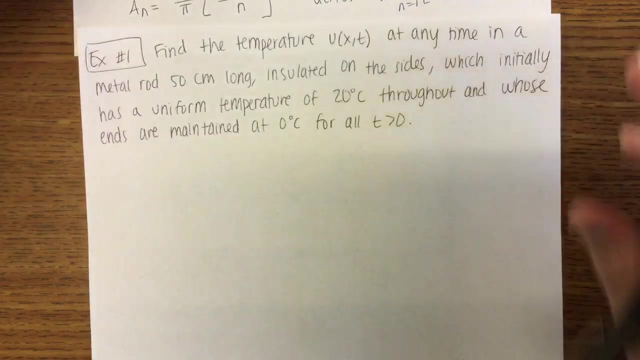 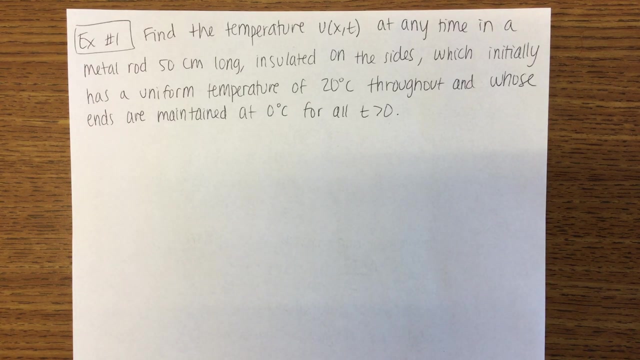 Has a uniform temperature Of 20 degrees Celsius throughout- Oh, that's a quick one, Mm-hmm. and whose ends are maintained at zero degrees Celsius for all T greater than zero Laterally. So that was one of the basic assumptions when we did the heat. 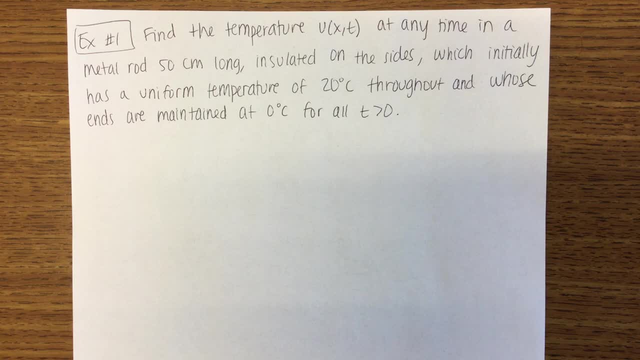 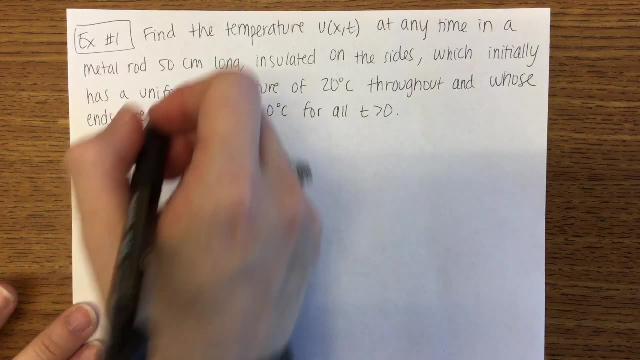 equation, because we're only going to be solving ones that are not losing or gaining heat of some type. Okay, first thing we want to do is obviously write what the equation and the conditions are going to be. So, starting with the heat equation, it's going to be K times the second partial of U with respect to X is: 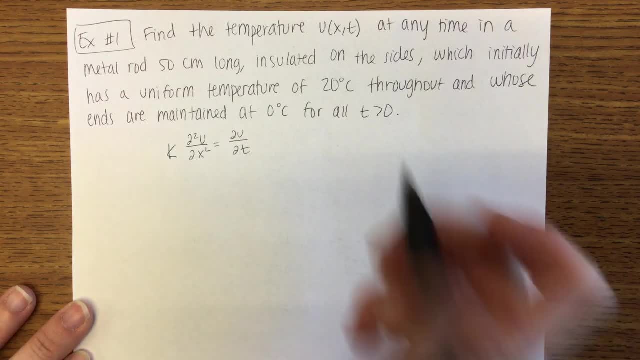 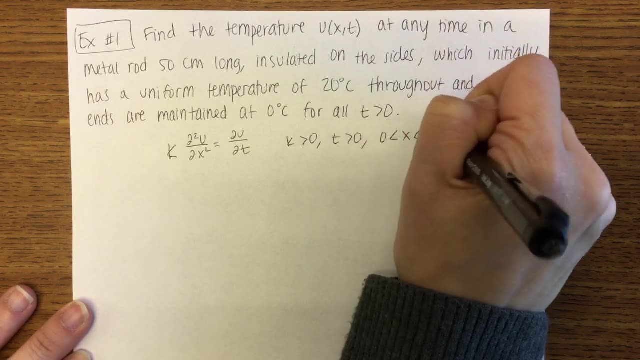 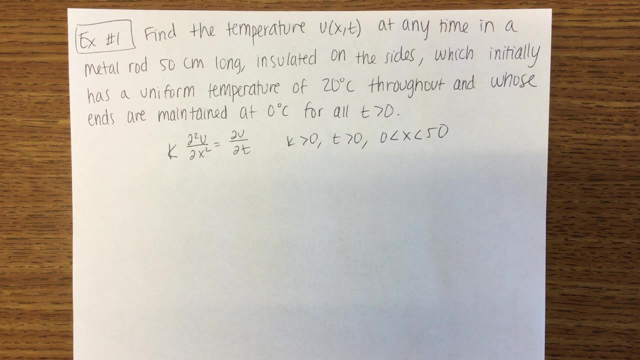 equal to partial of U. with respect to T, We know that K is greater than zero. we know that T is greater than zero. We know that X is between zero and, in this case, 50. Normally we would write L, but in this case, we know what L is. we know that L is 50. We know that there's a. 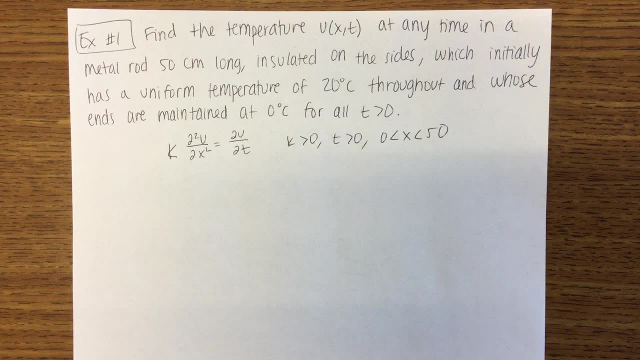 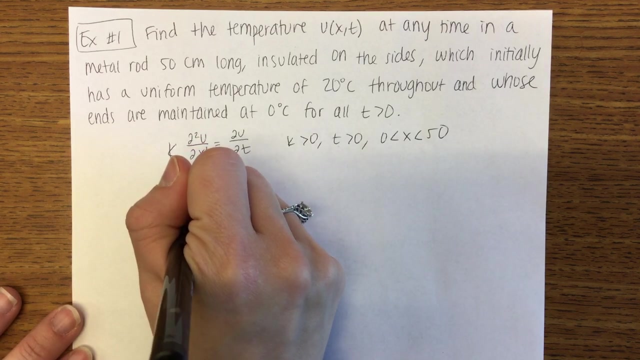 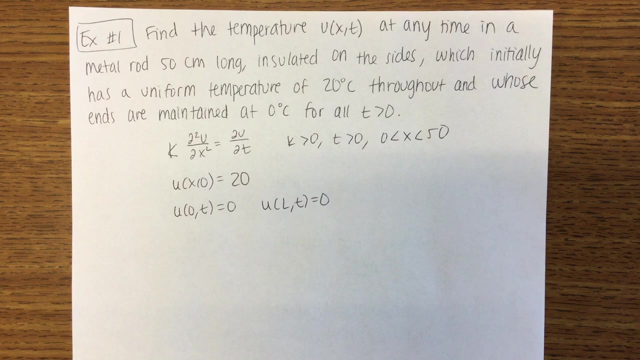 uniform temperature of 20 degrees throughout at the beginning. So that tells us that U, when time is zero, at every spot the temperature is 20.. And then we also know that the ends are maintained at zero degrees, so that tells us that U of zero- T equals zero and U of L- T equals zero. 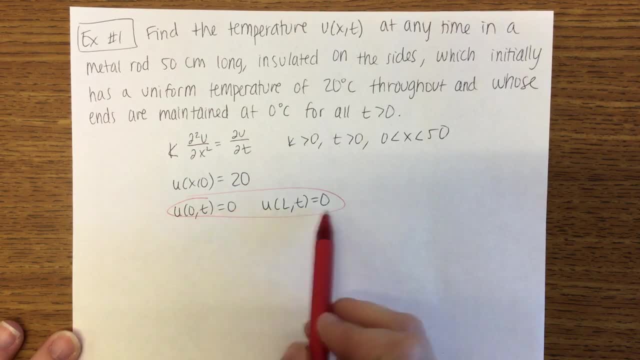 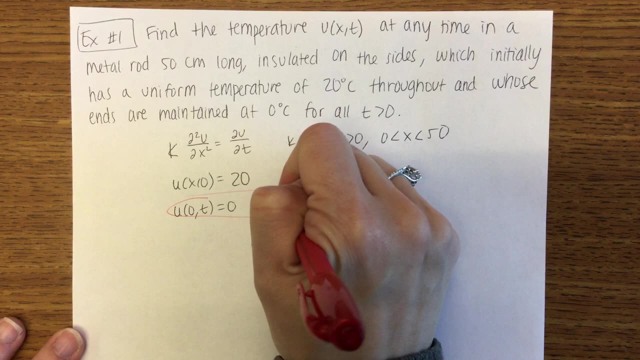 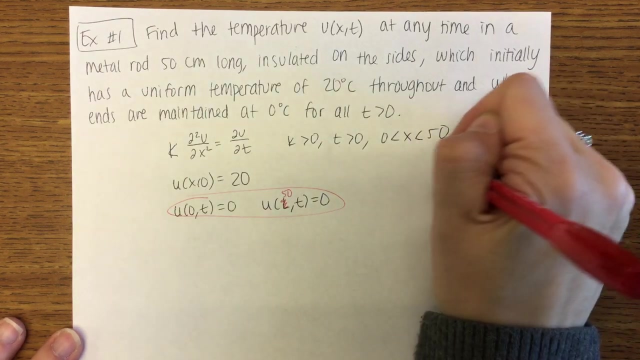 Okay again, this is the part that makes the equation homogeneous. Can you put 50 in there for L or no? Yes, I'm sorry, this should be 50, so this is also 50.. Since you gave 50 in the classroom, he has to found 20 too. 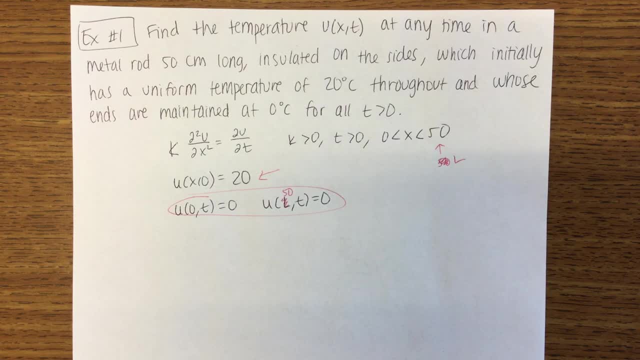 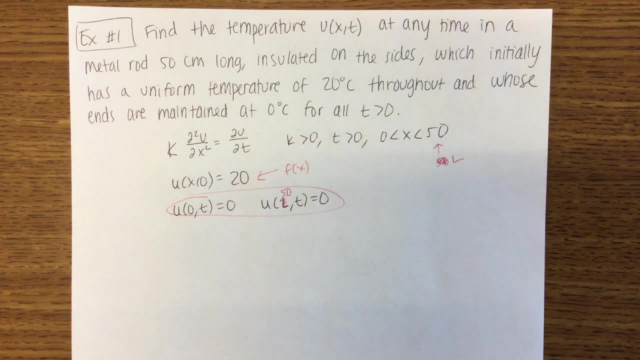 Well, he has to find this answer, right. Yeah, but since we're solving for X, we'd have to put the answer in their values of plus or minus L. Yeah, so five times W equals one. Okay, so now we have to get back out there first. 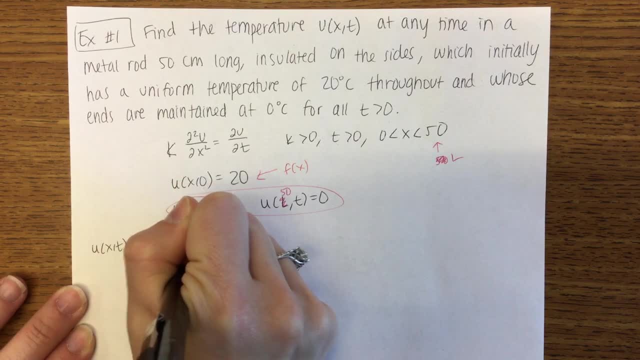 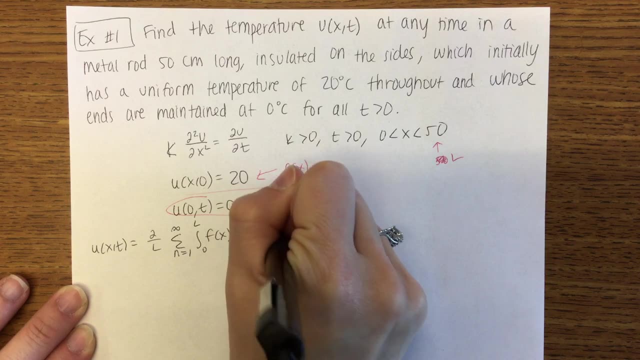 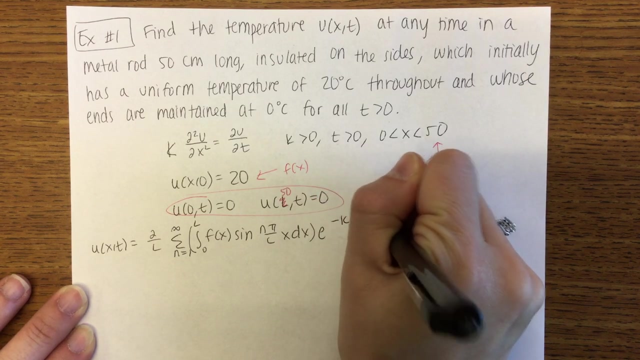 So we would have to get solving for L in order to say So. the answer to this is: it's going to be cross times X times L. timing markt: ok: 10 times X. sine of n, pi over l, x, dx times e. to the negative: k: n squared pi squared over l squared t. 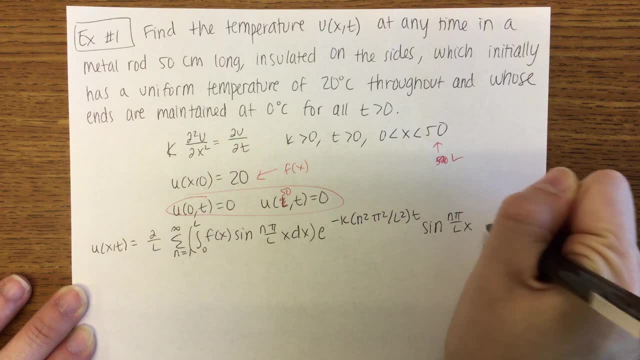 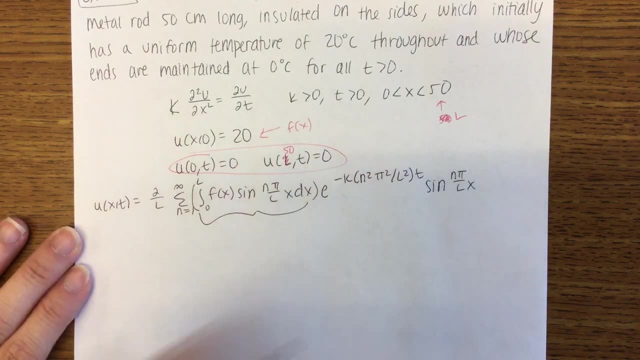 sine of n pi over l, x. So that's what our final solution is going to look like. We are going to start by finding this integral: Yes, I don't know. Okay, I don't know, That's what I'm going to do. 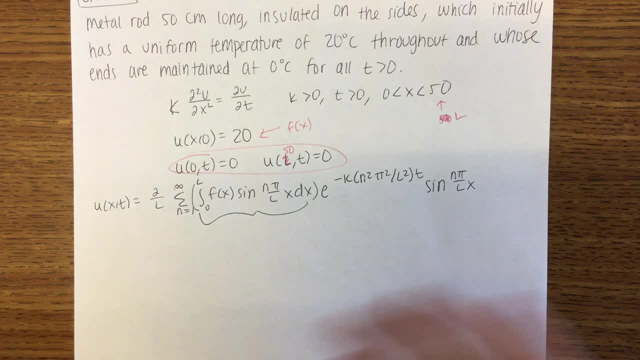 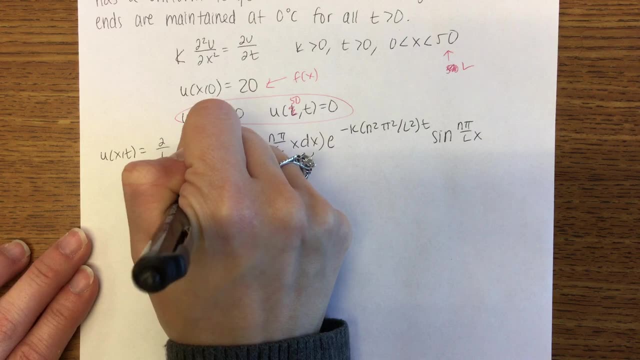 That's what I'm going to do. That's just how it is. Just accept it. okay. Ask your physics teacher later today. Okay so, this is going to be the integral from 0 to 50, because l is 50.. 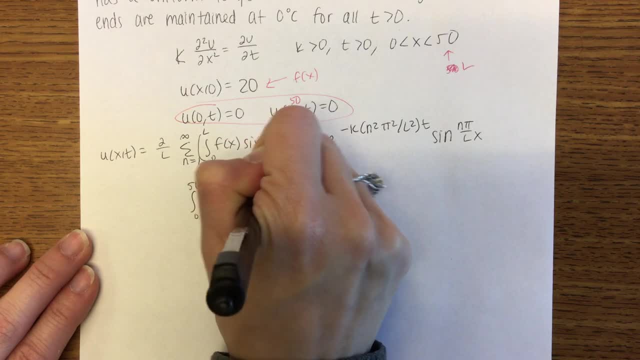 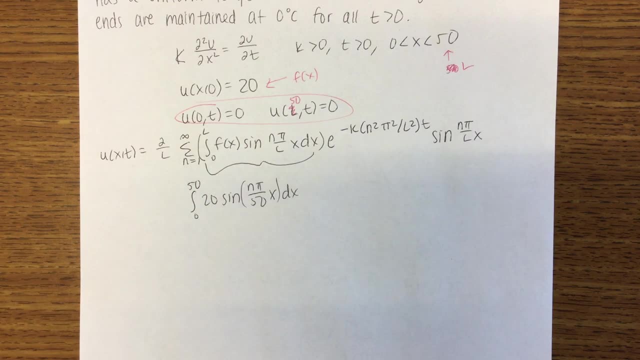 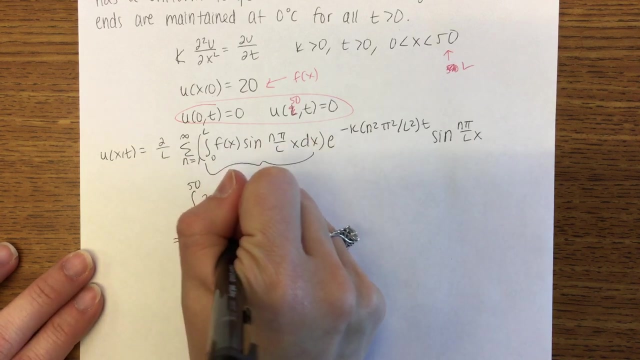 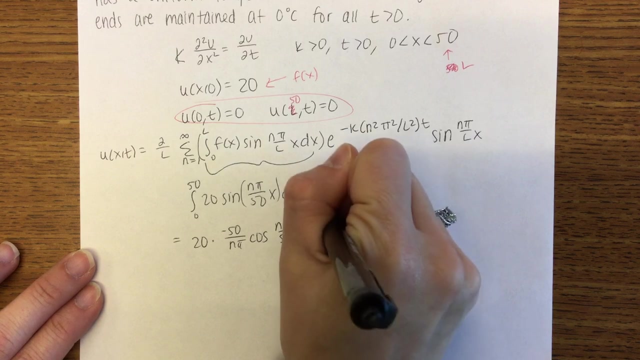 f of x, like we talked about, is 20.. This will be sine of n? pi over 50 x, dx x. So then we're going to be left with 20 times negative 50 over n pi. cosine of n? pi over 50 x from 0 to 50.. 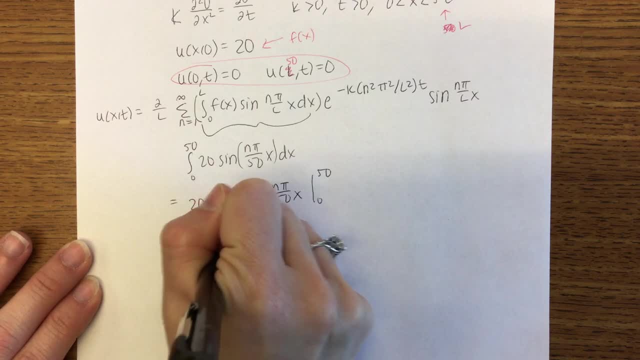 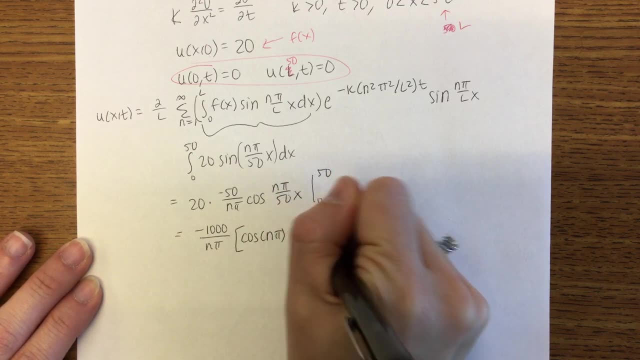 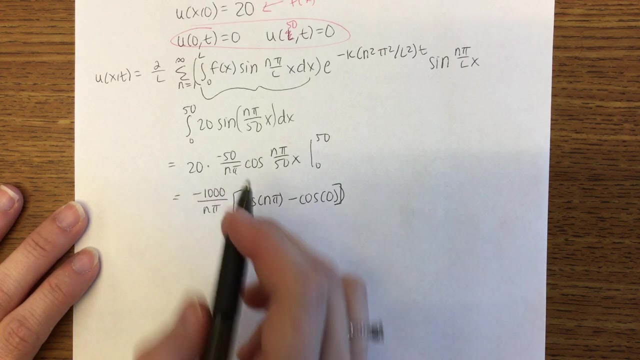 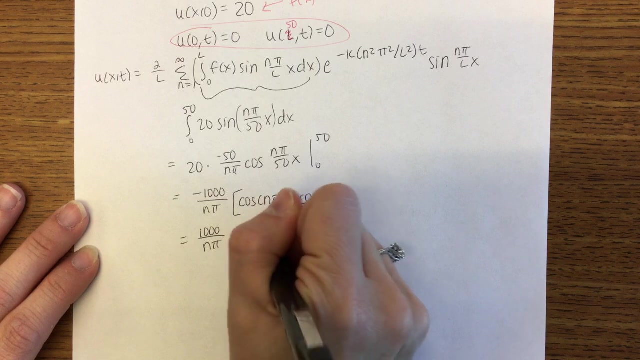 So this gives us negative 1,000 over n pi. If I plug in 50, I get cosine of n pi minus cosine of 0. I don't like the negative, so I'm going to switch this around to be cosine of 0 minus cosine of n pi. 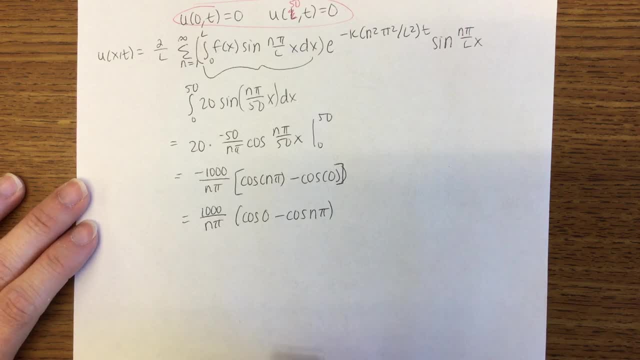 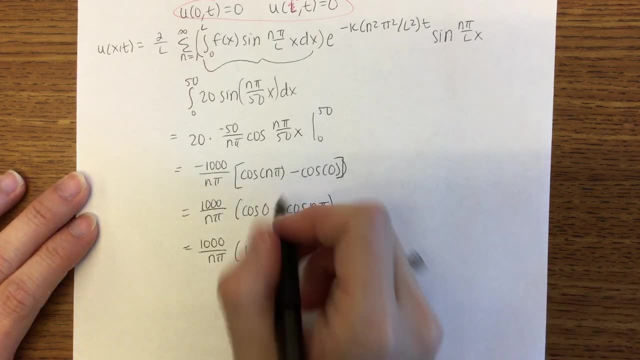 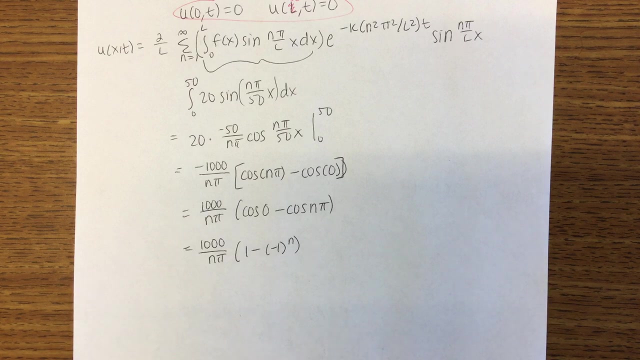 Okay, Cosine of 0 is 1.. We've already talked about cosine of n? pi is negative 1 to the n, And then cosine of n? pi is negative 1 to the n, And then cosine of n? pi is negative 1 to the n. 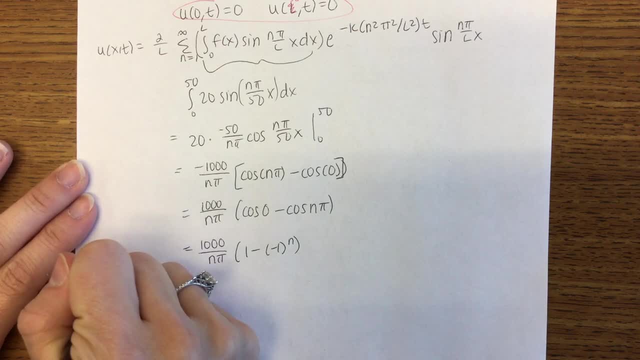 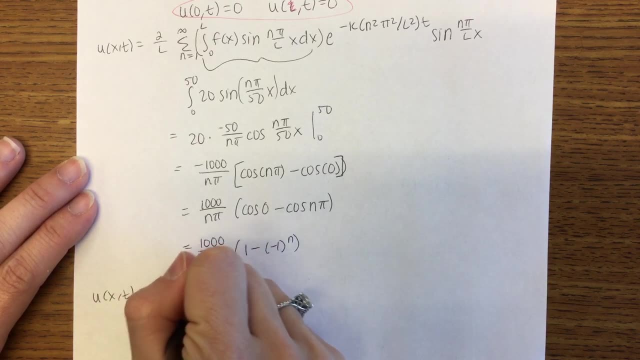 Okay, so our u of xt then It's going to be 2 over l, so 2 over 50.. Summation from n equals 1 to infinity of 1,000 over n. pi 1 minus negative 1 to the n. 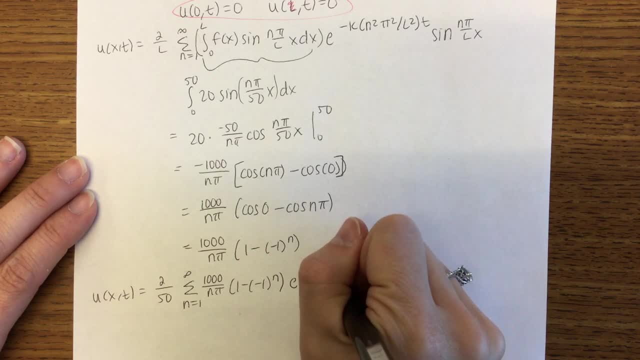 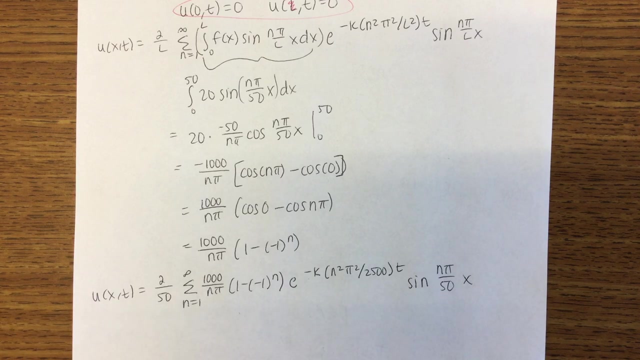 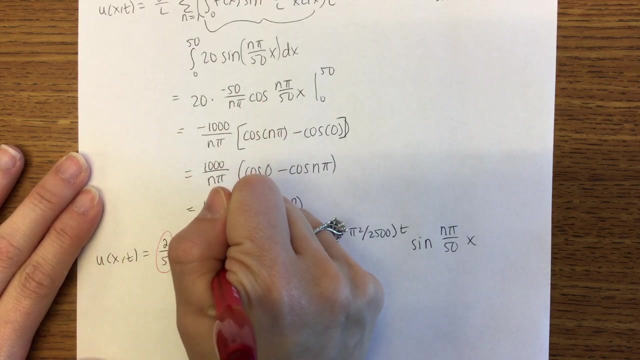 e to the negative k, n squared, pi squared over l squared, which in this case is 2,500 t sine of n, pi, n, pi over 50 x. Not how your answer is going to be written, though. You're going to combine those and the 1,000 over pi. 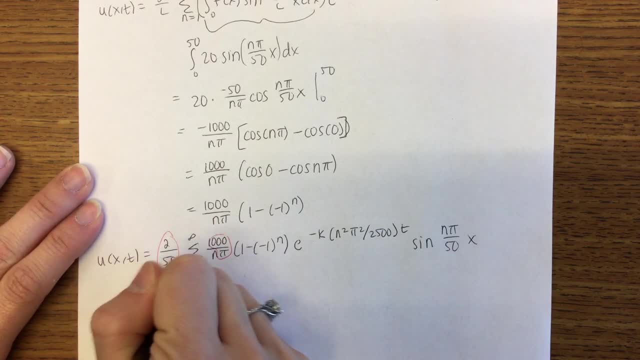 and of course you have to leave. So the final answer is going to be 40 over pi. the sum from n equals 1 to infinity of 1, minus negative negative 1 to the n over n, and then everything else like it appeared before. 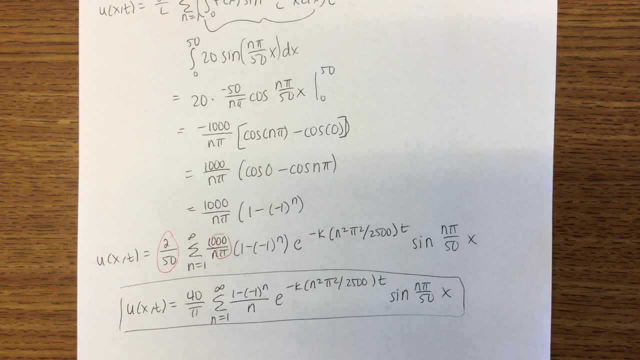 It's a constant of some type. No idea, Sorry, I would love to be able to tell you, but I don't know. Okay, questions on solving these Kind of yes, Okay. so here's what I'm okay with. 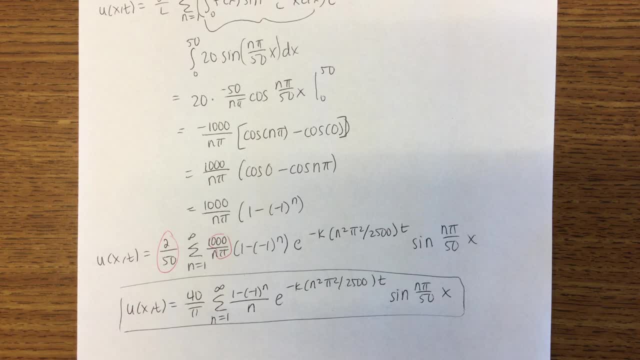 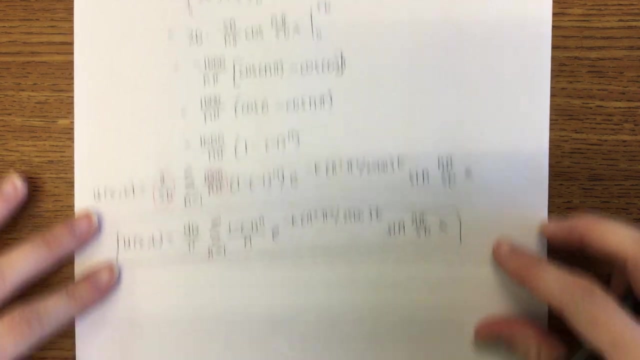 I'm okay with you using that equation If- A- you know how I got it and B- you have it memorized correctly. You do need to know the process, though, because you are also going to see an equation like this in your homework tonight. 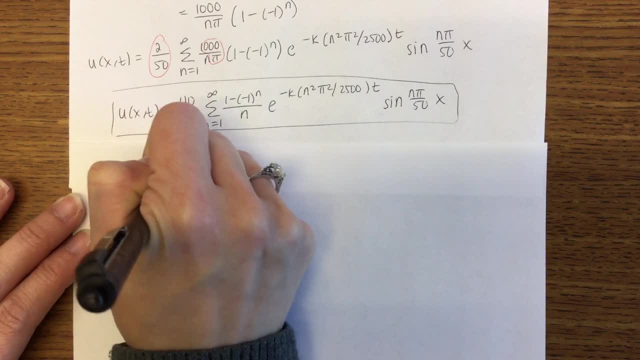 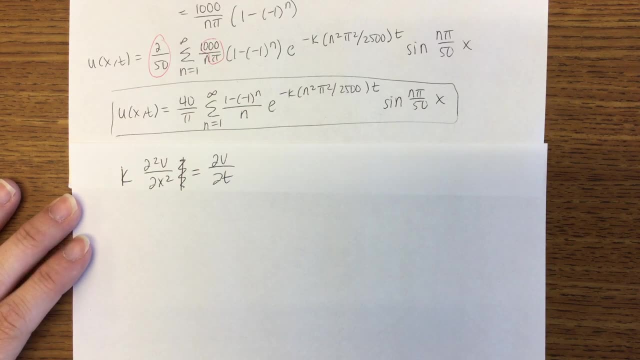 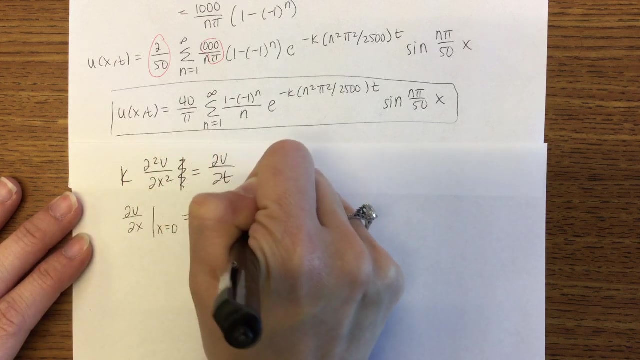 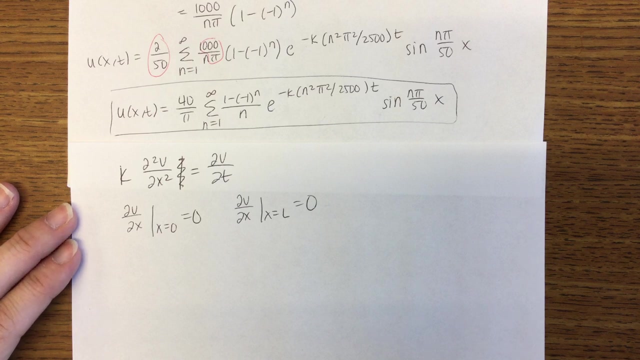 Or a problem like this in your homework tonight. Okay, so that part looks the same, but then these are the boundary conditions that you're going to be given, So this is no longer the equation that we started with. So in this case, you're going to have to derive a solution again, like we just did. 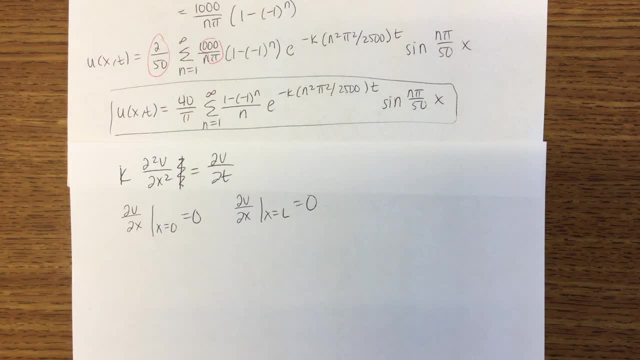 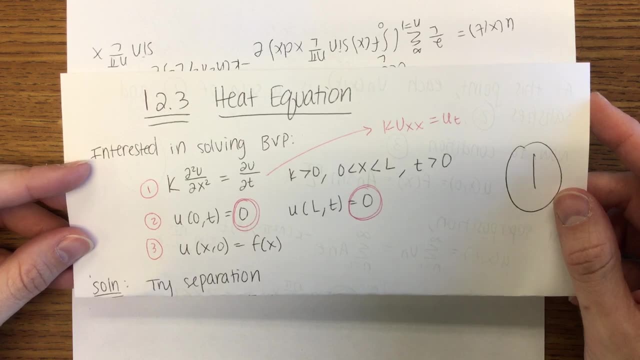 So if it looks exactly the same as what we started out with- which was this problem here- you can memorize the solution like we found it. Now, when we get to non-homogeneous, there's not going to be a nice solution that you can memorize. 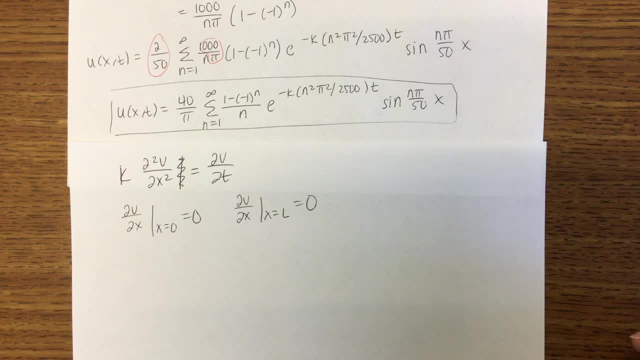 When we get to non-homogeneous heat and wave, you're going to have to do this process each time, And that's section 12.6, so that we're starting next week. So you do need to understand it, particularly when you get to this problem in your homework. 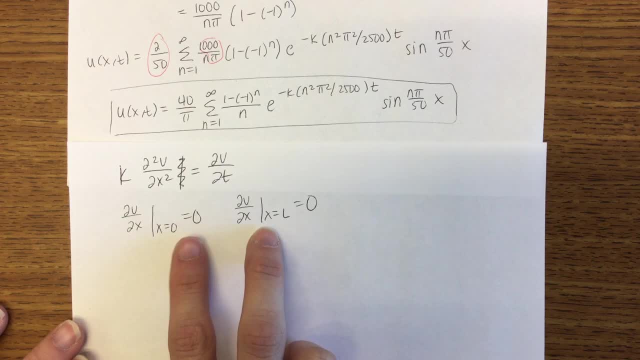 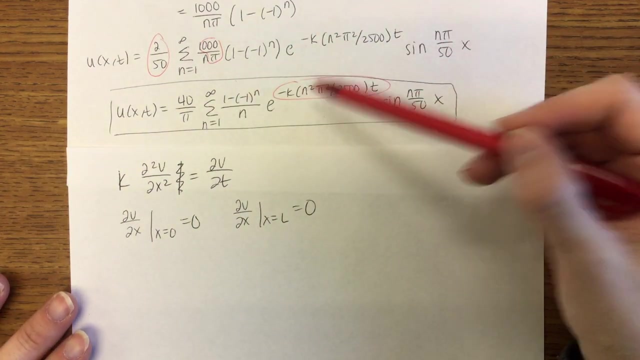 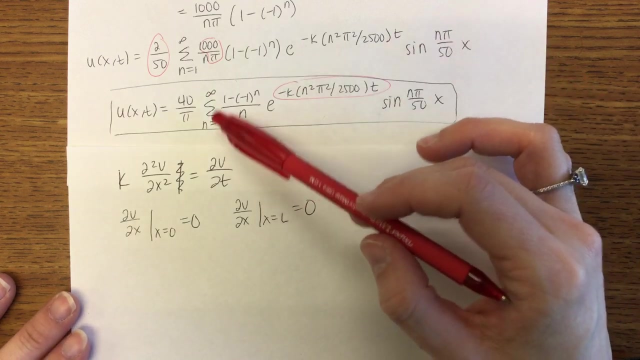 What do these mean? Ns are insulated. Okay, a few things to note. First, note this exponent as n gets pretty big and t gets big, we're going to end up converging. So ultimately we don't have to look at a whole lot of terms to get a pretty good representation. 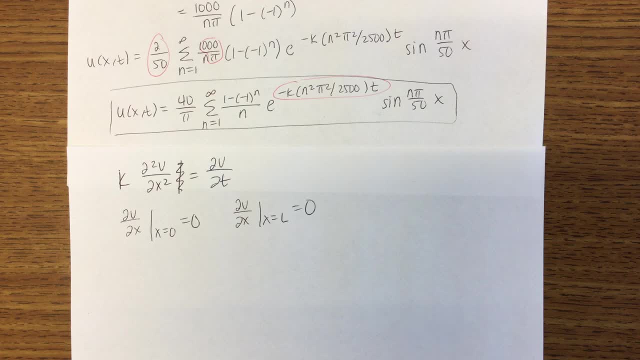 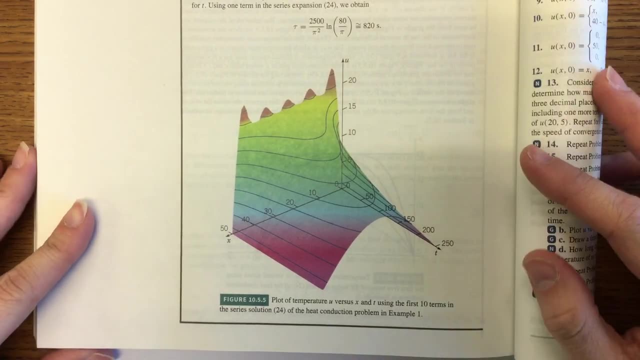 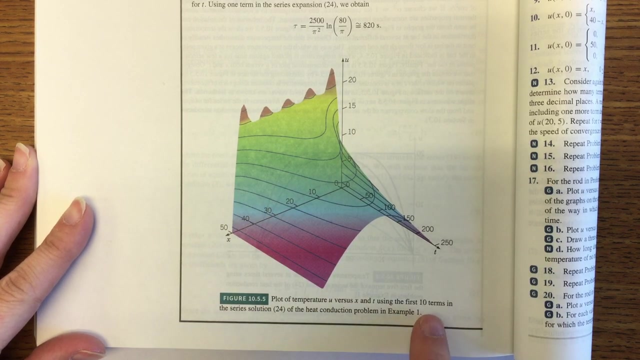 This is what people generally do, then, And we don't have the power to do this, But this is a 3D graph plotting space and time to find the temperature, Using only the first 10 terms. So they decided the first 10 terms were pretty good representation. 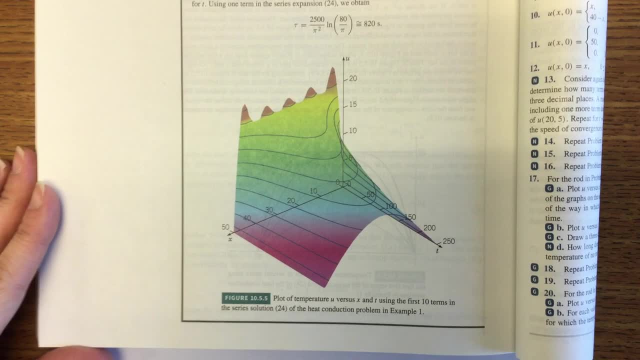 Sound good. Like I said, we don't have the power. 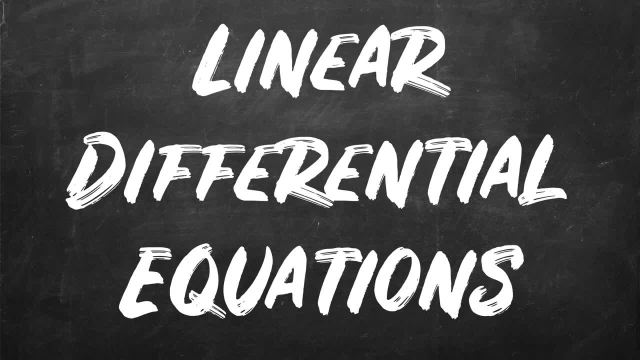 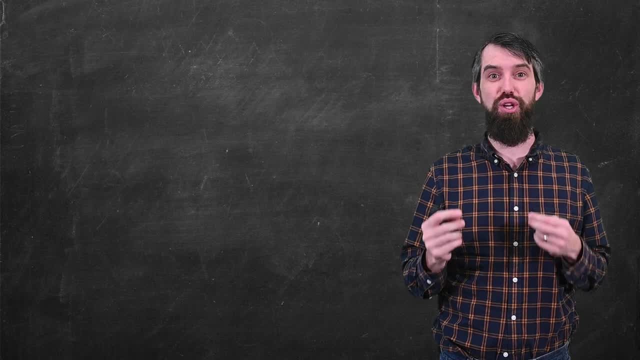 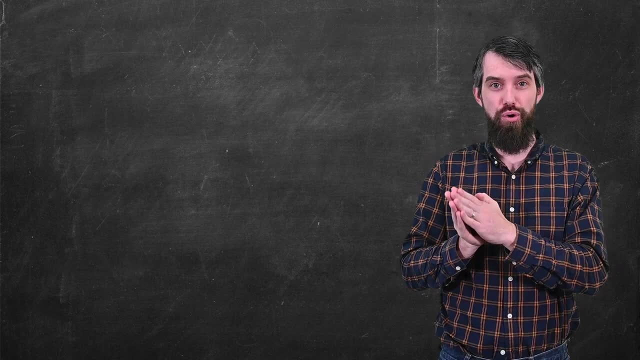 In this video we're going to study linear differential equations and, in particular, we're going to study first-order linear differential equations and the method of integrating factors, which is a wonderful way to always find a solution to a first-order linear differential equation. This video is part of my entire playlist on differential. 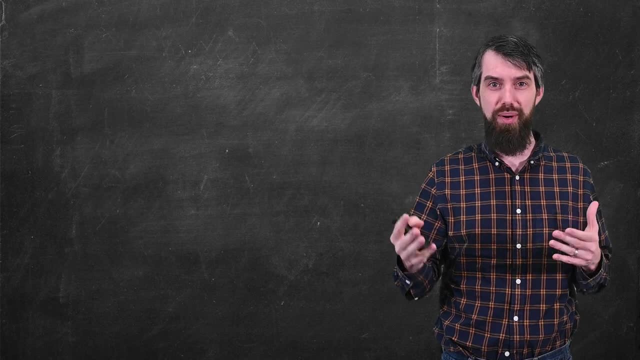 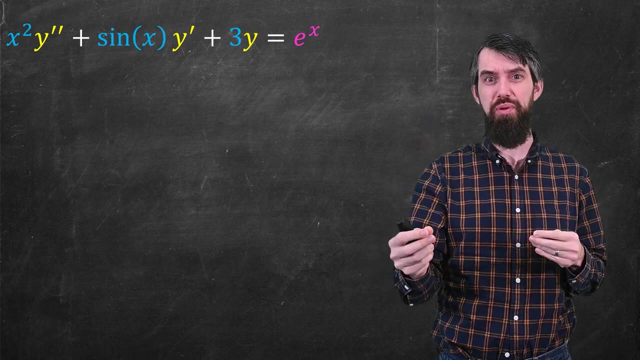 equations. The link to that playlist and the free, open-source textbook that accompanies it is down in the description. There is one heuristic that weaves its way throughout a lot of mathematics, which is that linear equations tend to be easier to understand and manage, and